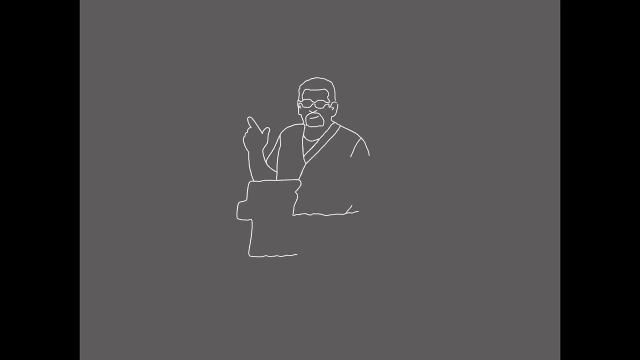 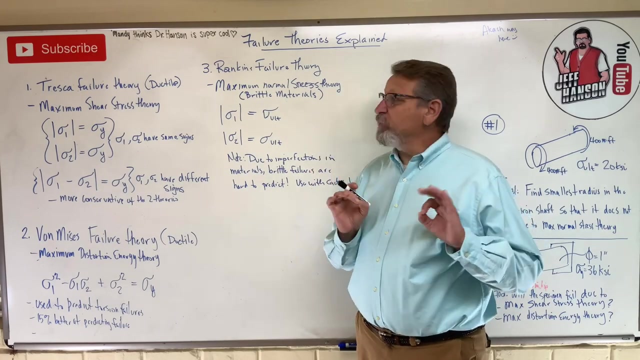 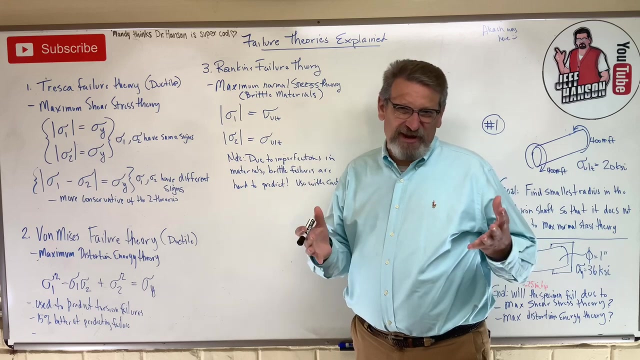 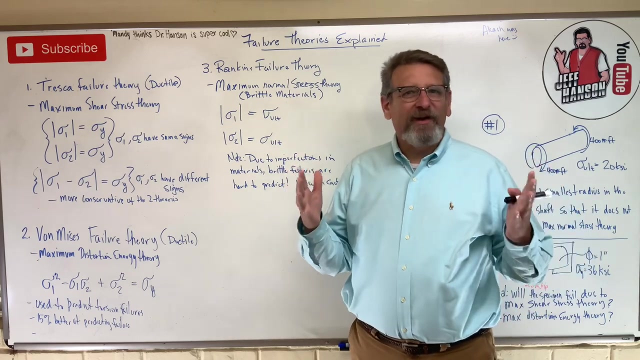 Hey gang, welcome back. Today we're talking about something that's a little bit tricky- failure theories- and I'm going to see if I can't explain this in a way where they're not so scary. okay, So when we're talking about failure theories, first off, what is a failure Now for us? 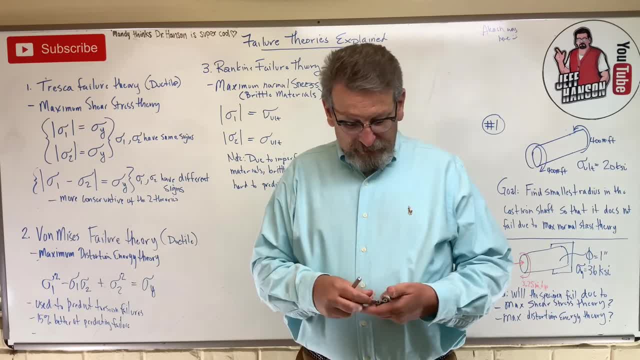 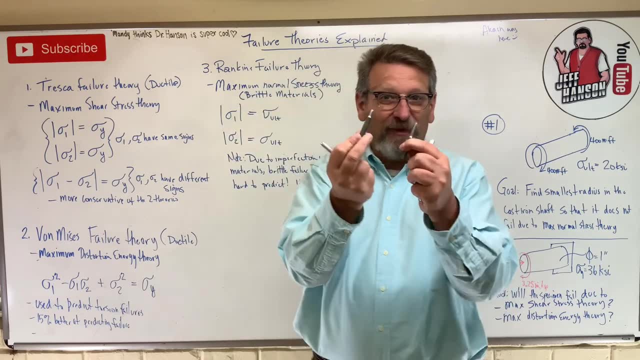 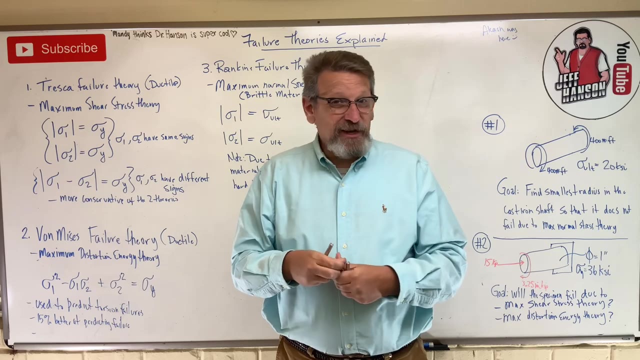 engineers, anything that's a failure, you know. what you think about is if I have, you know, a sample of material and then once I pull on it too hard, pow, it breaks right, And now I have two pieces and we consider that to be a failure. But is that necessarily a failure As engineers? 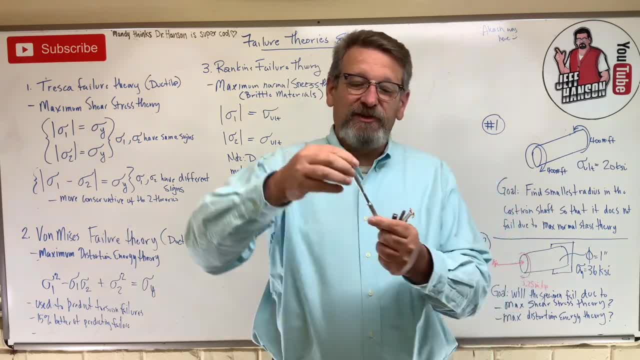 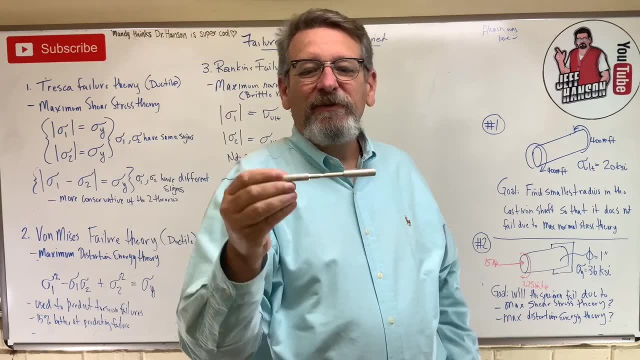 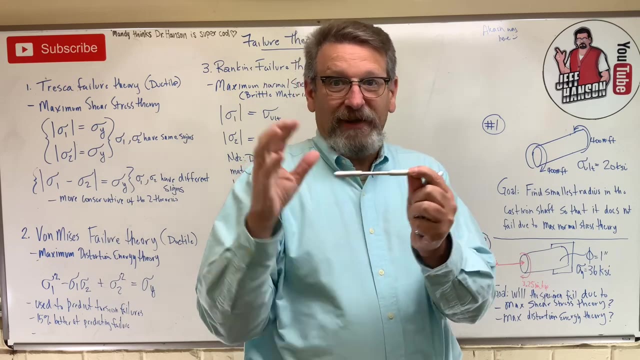 we don't. like. you know, I can't think of a whole lot of things that we design that are meant. look at that piece there. Can you see the center of it? Okay, the center of this is deformed. right, This has been stretched hard enough that this has yielded, right, It didn't go. 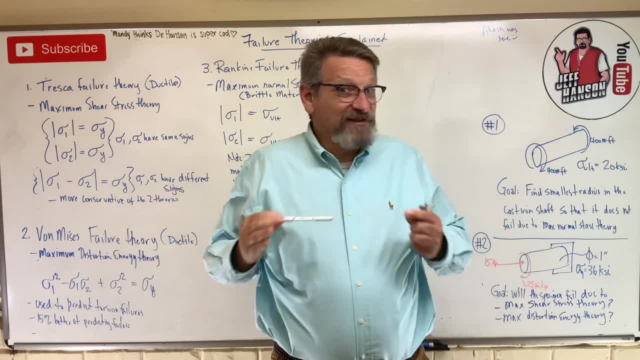 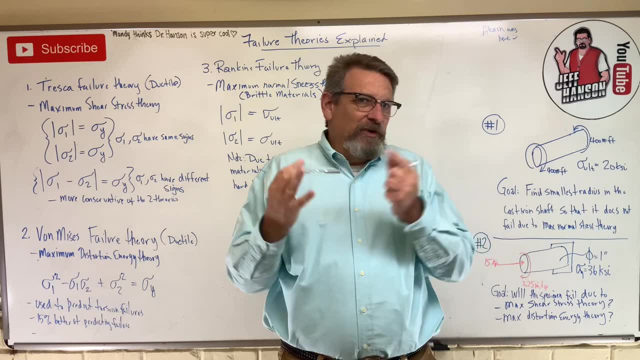 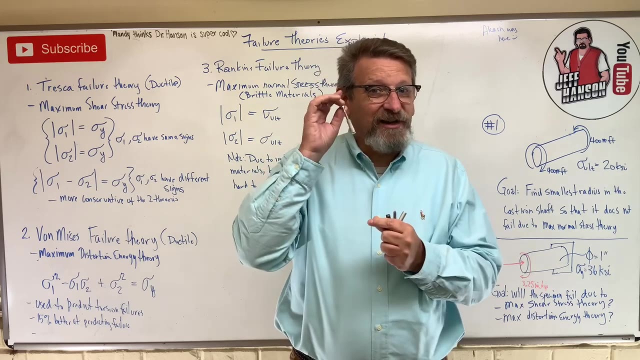 back elastically to where it started from. Is that a good thing? Can you think of anything that's supposed to yield and not go back, and then we can reuse it again? I don't know, you know. So failure for engineers does not necessarily mean ultimate strength, right? 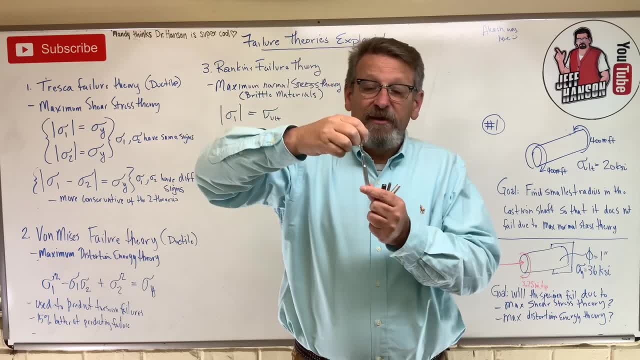 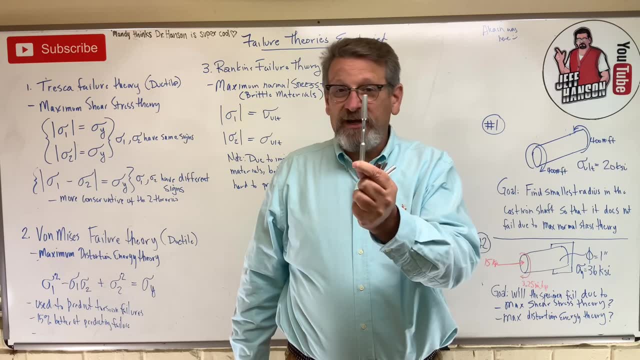 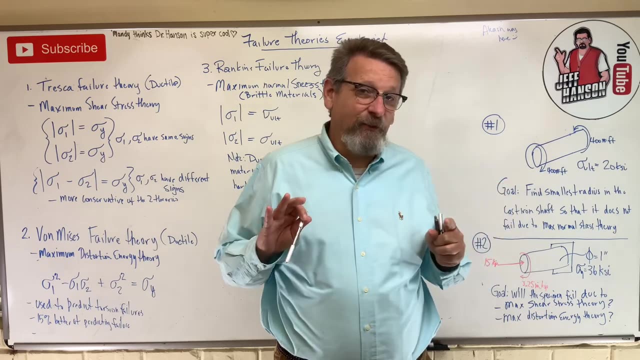 Not ultimate strength but fracture right, Two pieces. Failure to us can mean it has gone into the yielding portion of the curve there and it is elastically stretched beyond where it can't go back to where it started from. So generally as engineers, that's a no-no right. We don't want that. We don't want it to be. 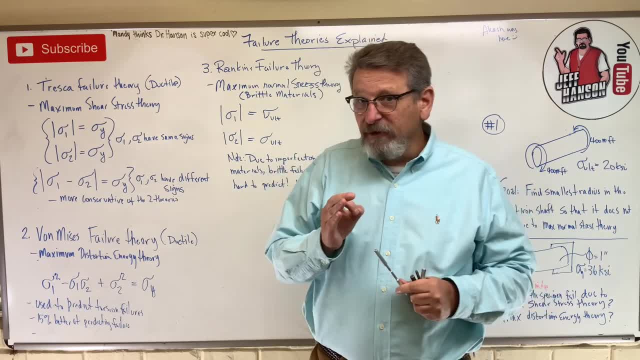 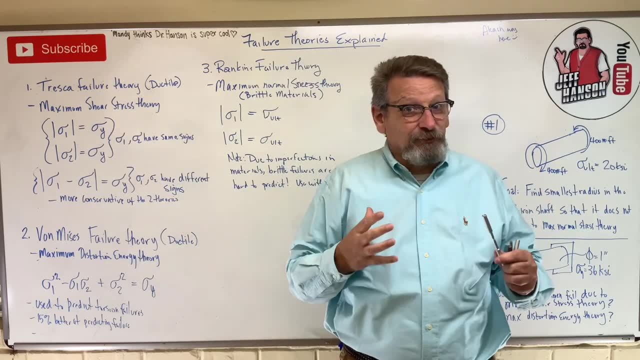 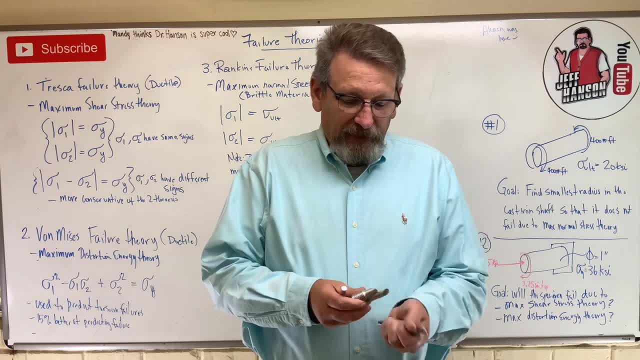 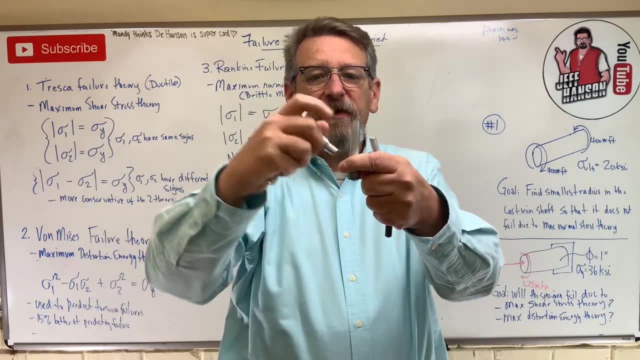 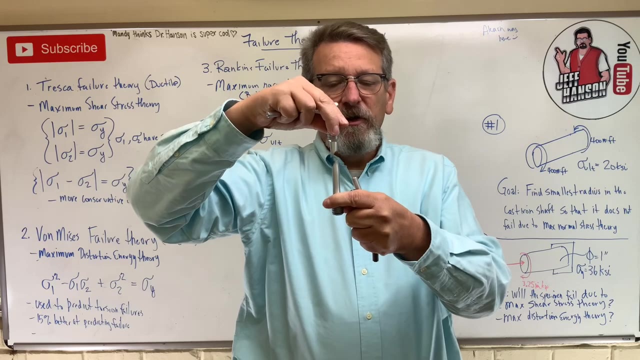 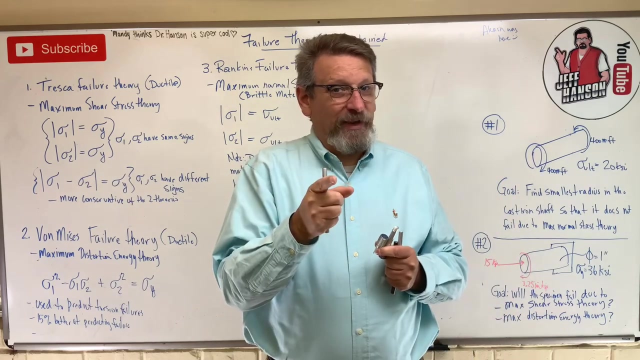 fail. remember you have a couple of things: typically brittle materials, right? brittle materials, when they fail, will fail on a 45 degree angle plane. look at that, 45 degrees, right, that's from shear. where does shear maximum occur, right? well, remember, in more circle we got a double the angle right and tau max is at 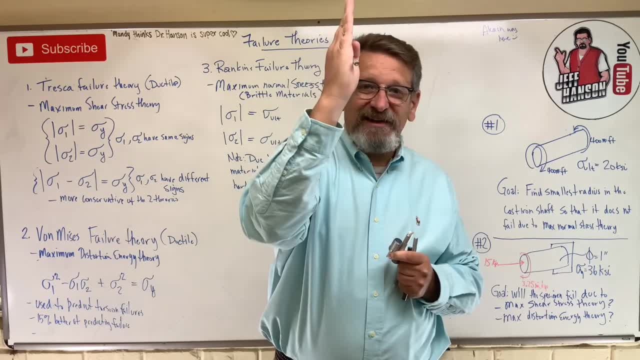 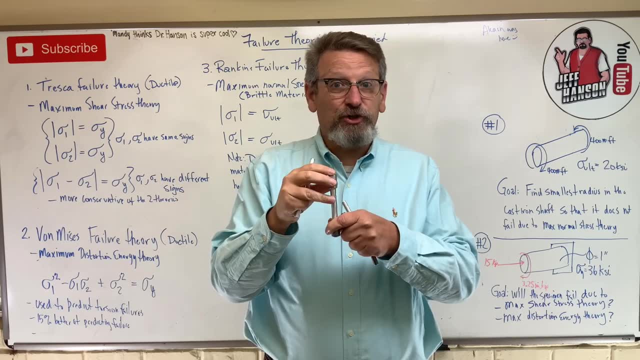 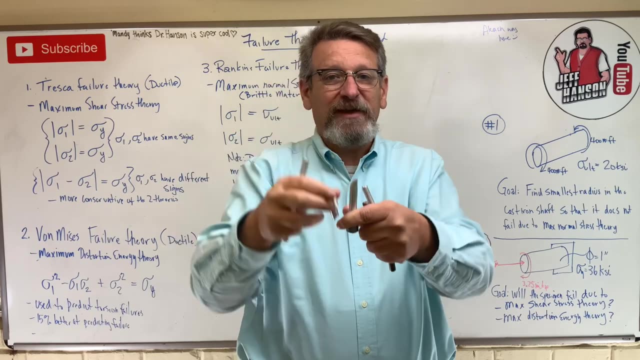 the very top of the circle right, which is 90 degrees, but in the real world that's 45 degrees. so at 45 degrees that, that shear stress is the very highest. and when it shears in half- look at that- it tears on a perfect 45 degree angle. 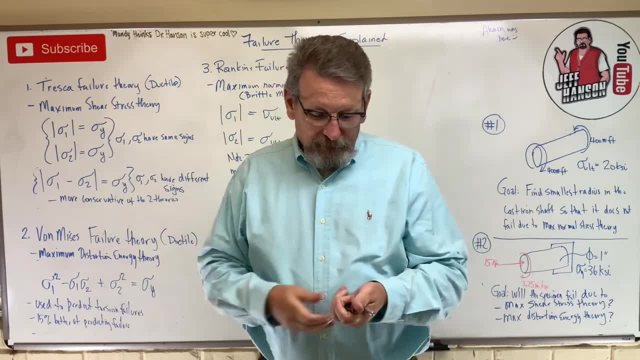 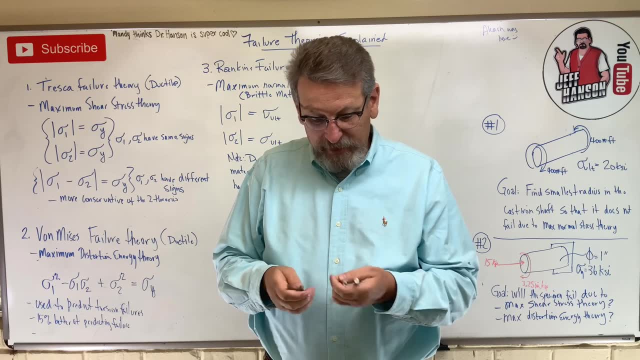 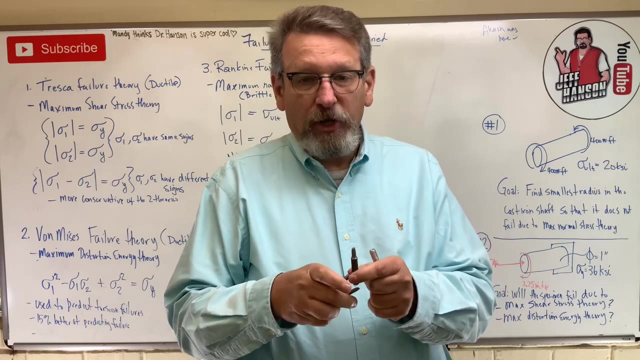 isn't that cool now for ductile materials. they don't tear exactly like that on a 45 degree angle. I don't know if you're gonna be able to see this or not, maybe. I've got a few examples here. this one's a little bit better. they fail on what's called a cup and cone. 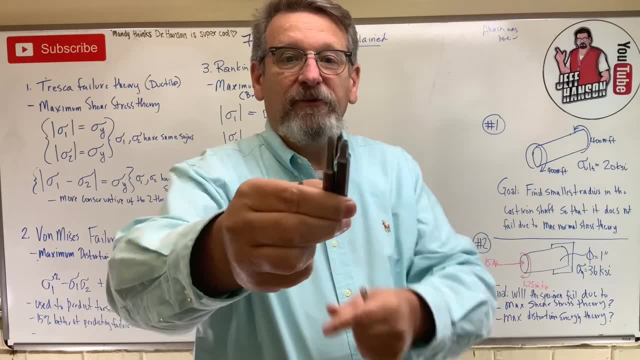 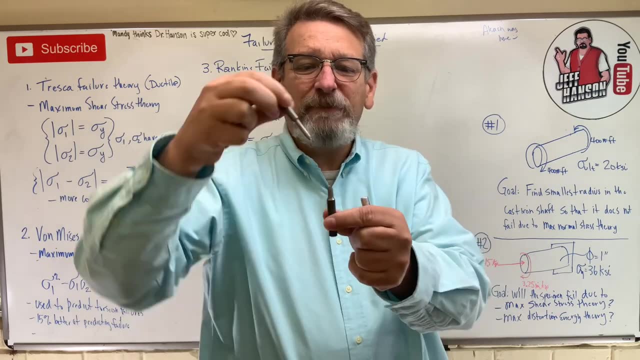 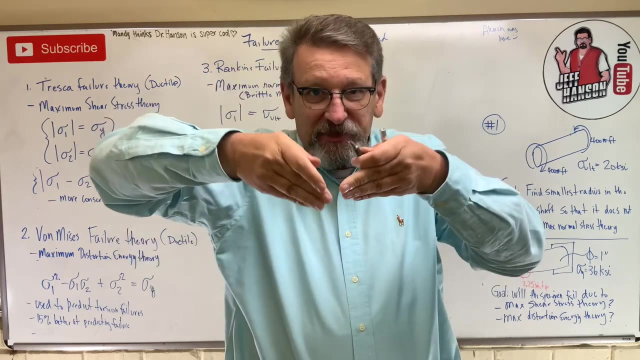 failure. okay, so I don't know if you can see this or not. okay, but one side, one side of this specimen fails in a little v-shaped cup and the other side of the specimen that pulled apart has a little v-shaped- the negative part that goes. that goes into that. right, these are all little test samples that we pulled apart. 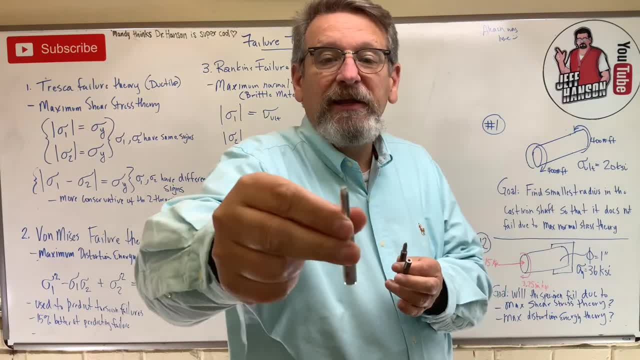 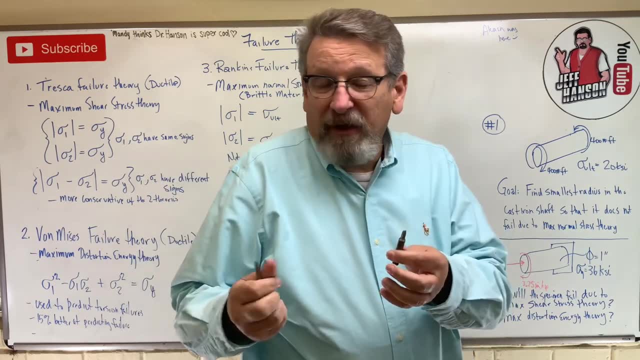 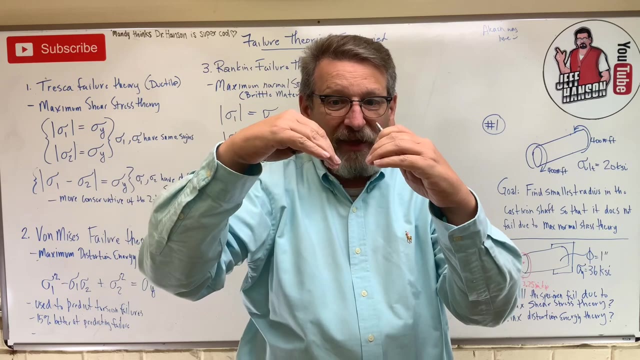 in the lab. okay, this one has a pretty nice- it's a little piece of aluminum- pretty nice little cup in there. but anyway, what's happening there? well, really and truly, it's failing on a 45 degree angle to. that cup has 45 degree angle sides, right, but it has it in all directions at the same time. and 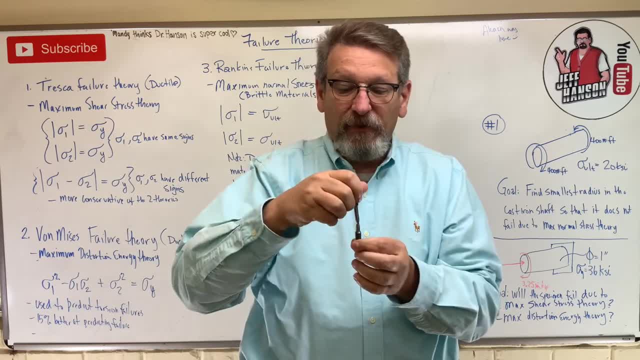 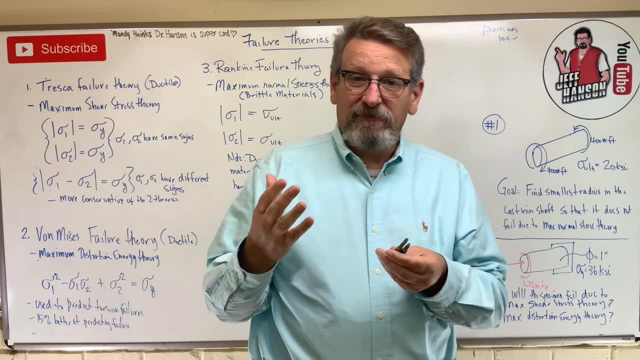 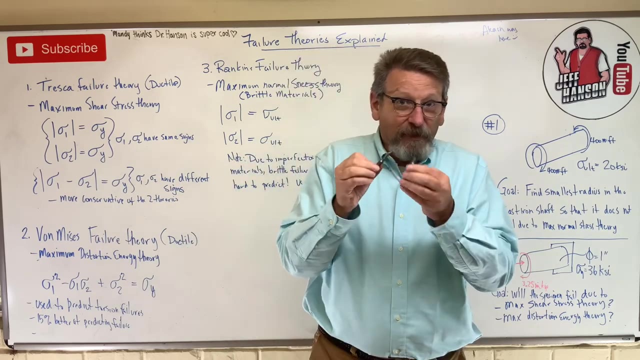 that's what makes that little cup in there. as that fail, and once we learn more circle that were tau max is straight up and down, it really makes sense that, hey, the sheer stress is the greatest at 45 degrees. and so when you look at these failures up close, they start to make sense. okay, and so what? 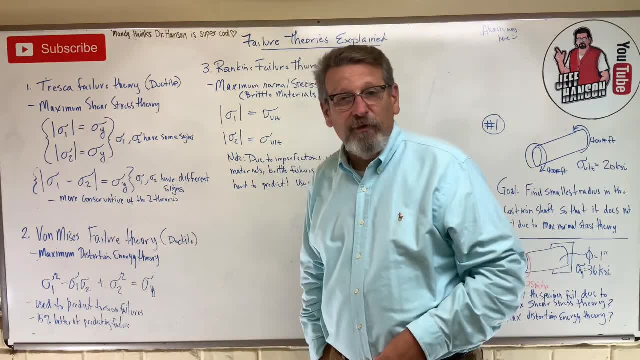 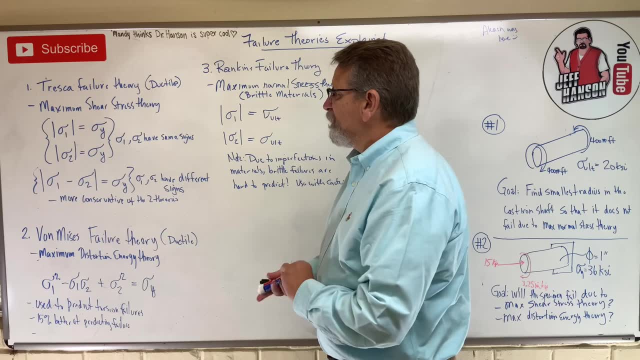 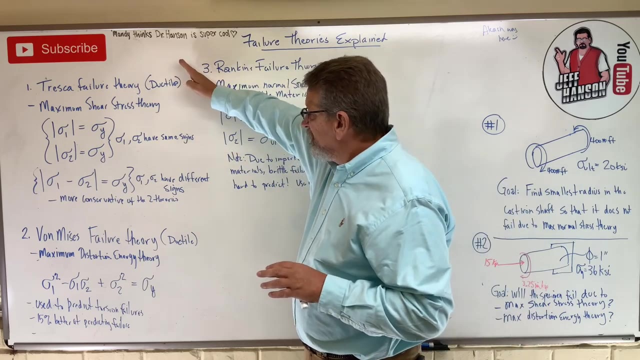 you've got here, what I have is a pocket full of broken parts. now, okay, anyway. so we're going to talk about some of these failure theories, okay, and we have basically two families of these failure theories. one is for ductile materials, and that would be the Tresca and the von Mises, okay, and the third would be the 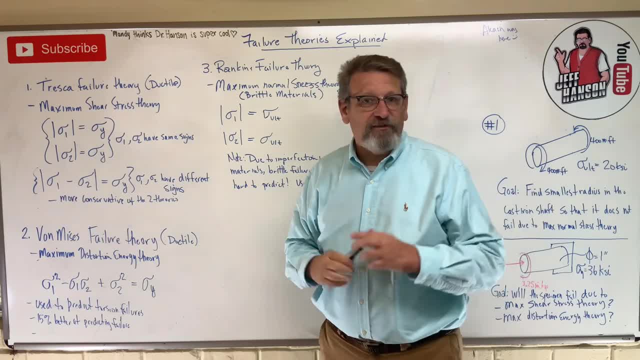 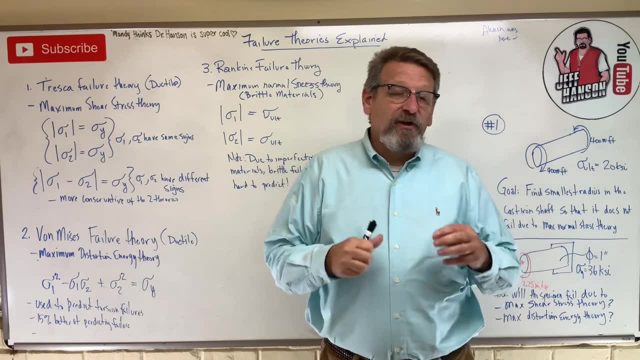 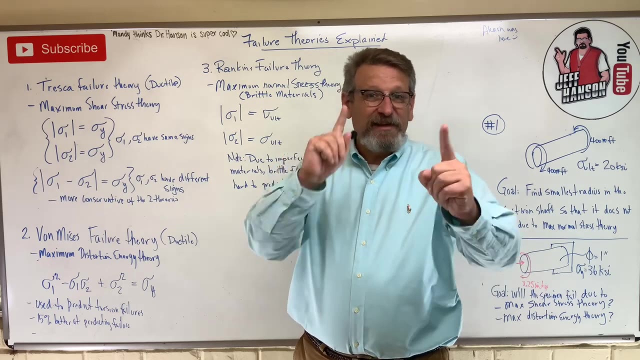 Rankine, and that would be for brittle materials. okay, we're going to talk about both of those and then we're going to work an example problem that uses these failure theories to tell whether we think a part would fail or not. and remember, fail does not mean break in half, fail means I've exceeded yield. strength. okay, so the Tresca failure theory is also called the maximum shear stress theory. these two things are the same. so Tresca and maximum shear stress theory- same thing, okay. Henry Tresca came up with this and he says this: that Sigma 1, the absolute value of Sigma 1, is equal to the Sigma. 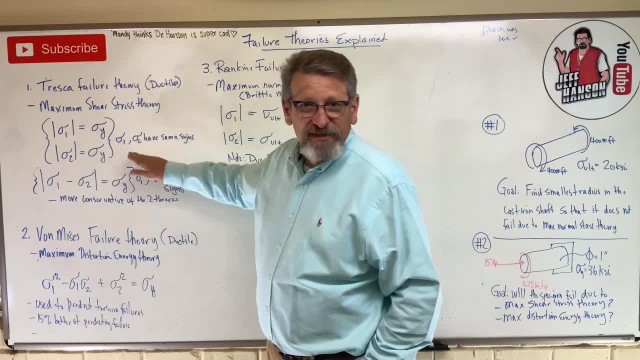 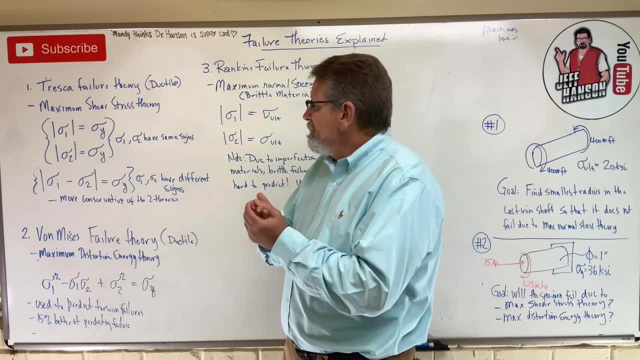 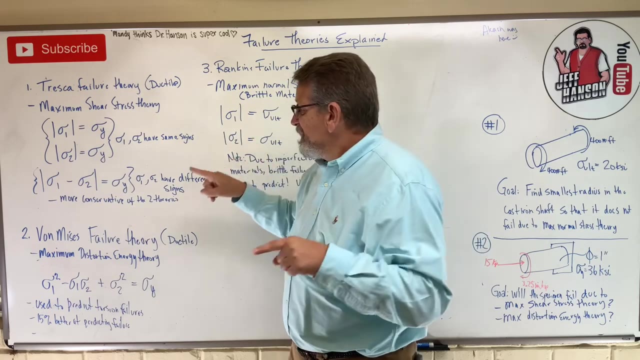 yield. okay, now this is what is Sigma 1 and Sigma 2. what is that? that's principal stress. how are we going to get principal stress? this sounds like the perfect job for a Moore circle, doesn't it? because we can get those two principal stresses, and then we? what this is basically is doing is comparing the 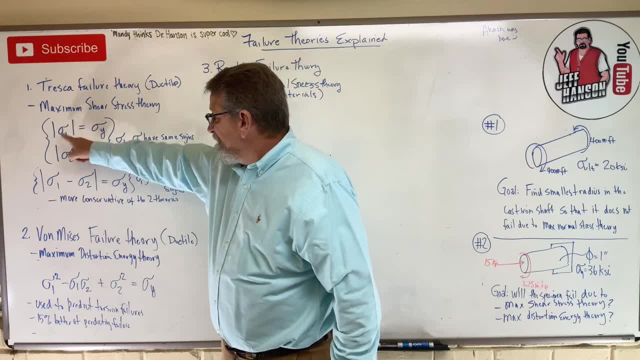 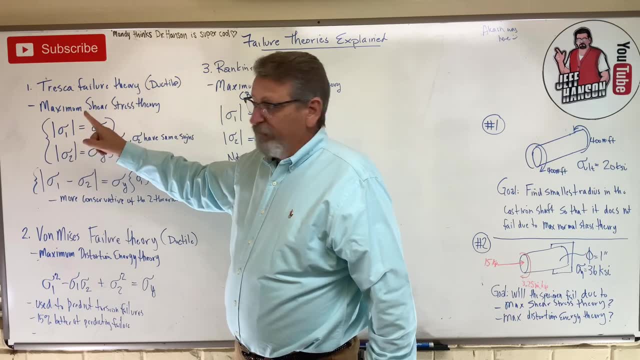 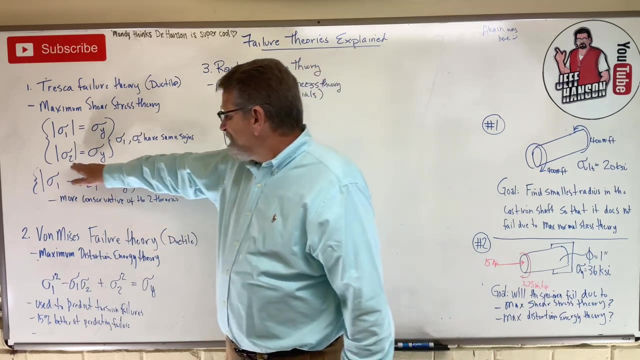 principal stress to the yield stress. if this guy is bigger than the yield stress, then we have a failure. if this guy is smaller than the yield stress, then it's not going to fail. okay, so this really isn't an equal. it should be a less than equal to there. and then, why is it Sigma 2? why are we checking that? well, remember. 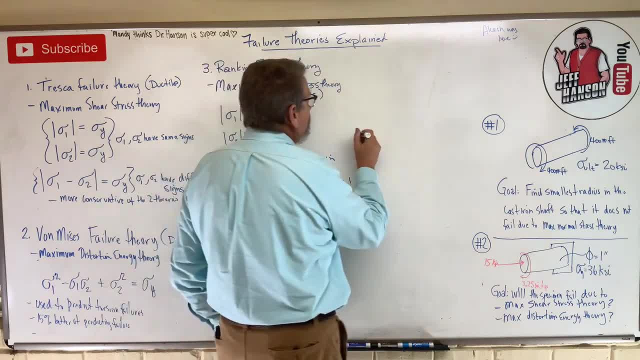 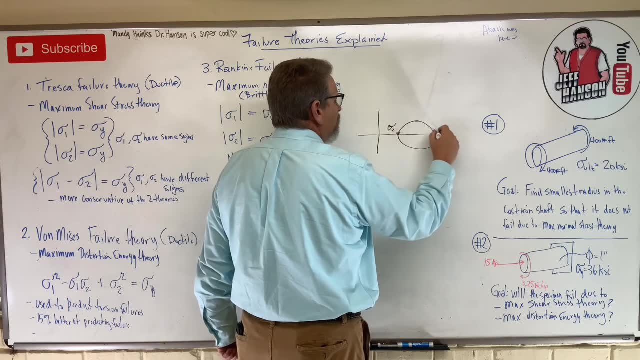 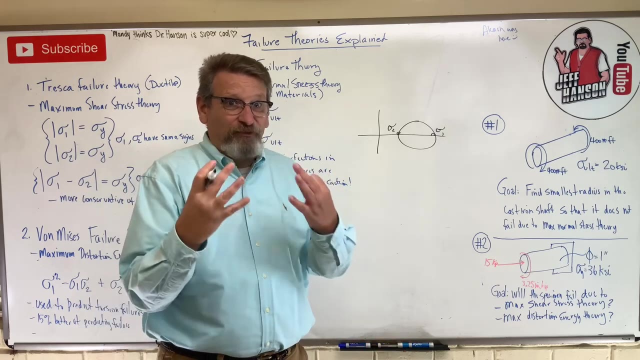 we have more circle. let me draw you a picture. sometimes we have more circle like this: okay, here's Sigma 2, here's Sigma 1. okay, who's biggest? Sigma 1, right, Sigma 1 is biggest. it's the absolute value. of Sigma 1 is bigger, right, but 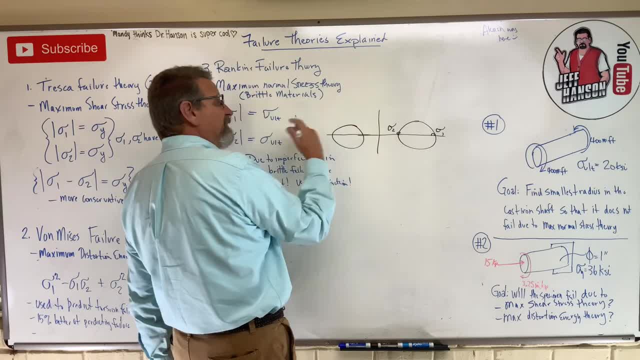 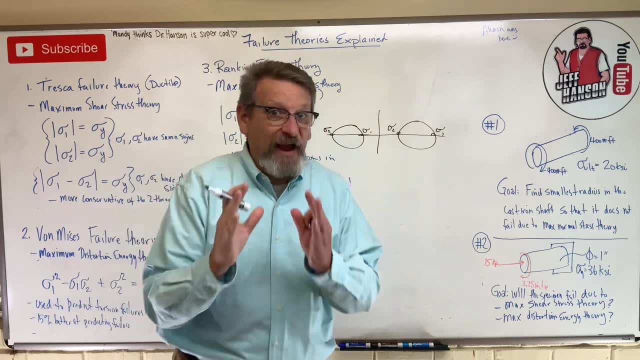 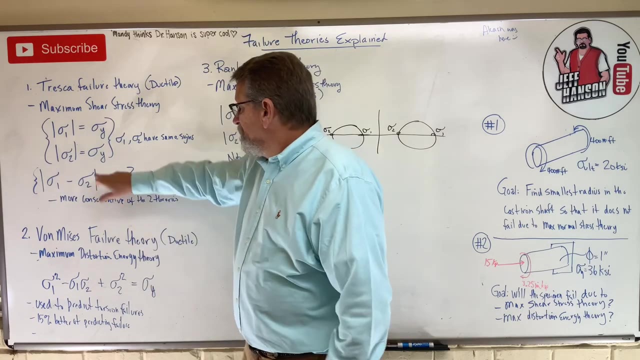 what happens if my circle is over here, on this side of the axis. now, here's my Sigma 1, here's my Sigma 2. now, if we're talking absolute value, right, well, now, Sigma Sigma 2 is a bigger number, right? so Sigma 2 is. we would use that. basically, what is it we'll use? 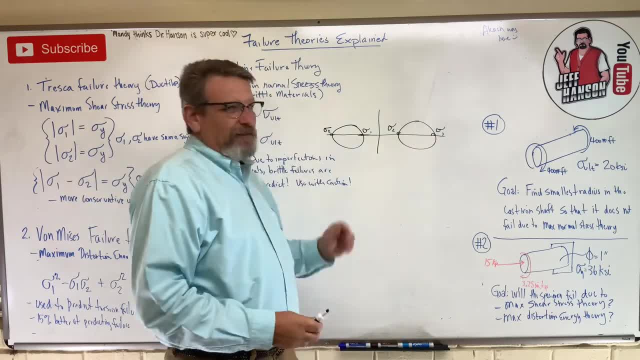 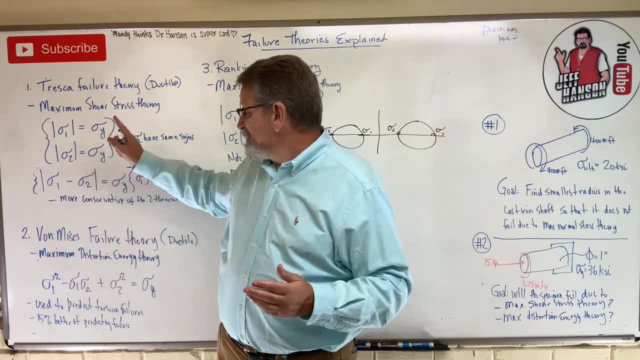 Sigma 2 when Moore circle is on that side and we'll use Sigma 1 when Moore circle is on that side. does that make sense? so whoever's absolute value is bigger, that's the one we're going to use, okay, so I hope that makes sense. why? 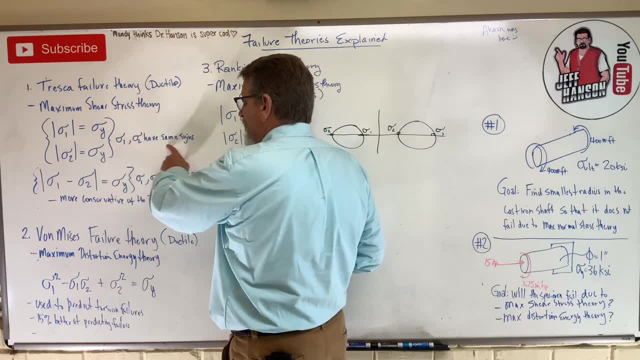 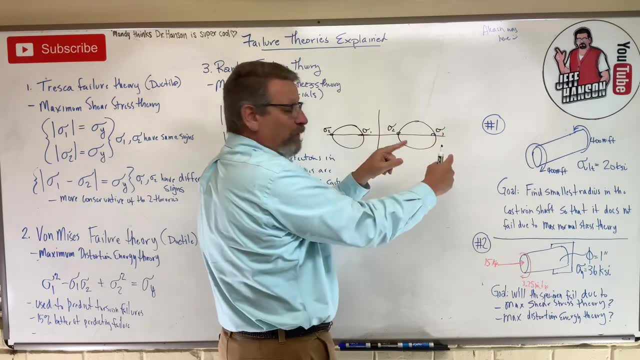 that's that way. so that's why it says: when Sigma 1 and Sigma 2 have the same signs, which means that that circle is completely that way, that's positive, that's positive. when the circle is completely this way, that's negative, that's negative. right, then we would use that first option there, okay. 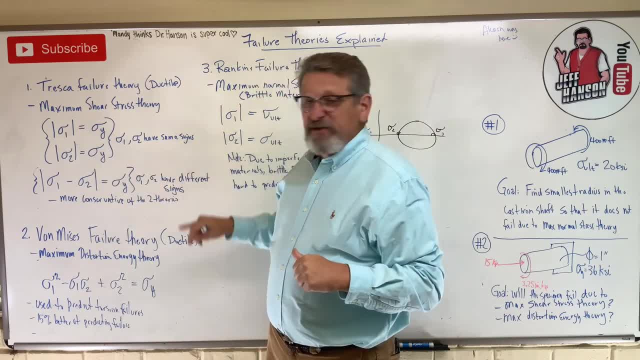 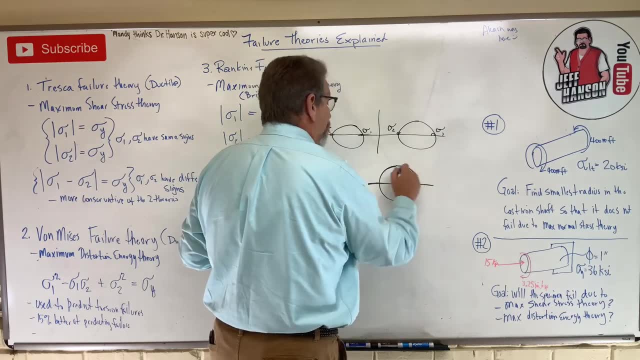 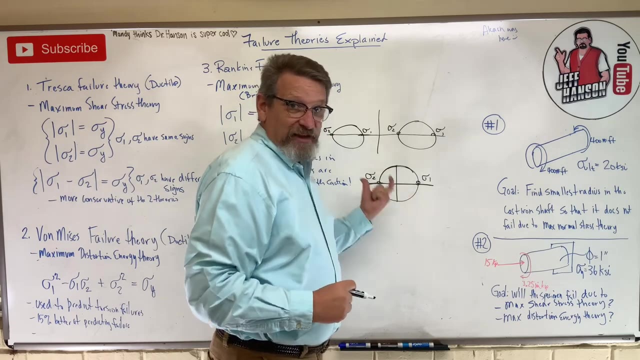 now, if what down here it says they have different signs, when would they have different signs? well, that would be a Moore circle that straddles the axis, okay. here's Sigma 1, here's Sigma 2. so if you have a Moore circle that straddles the axis, okay, then you have to do this, you have to take the 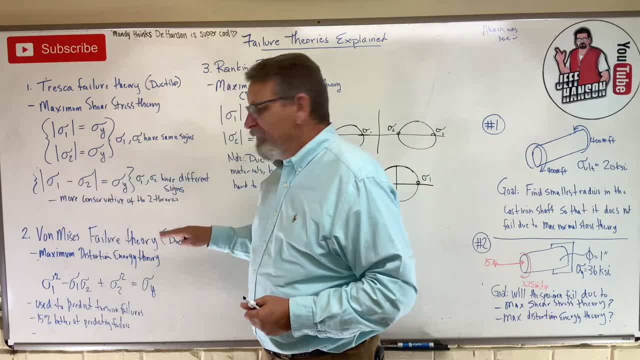 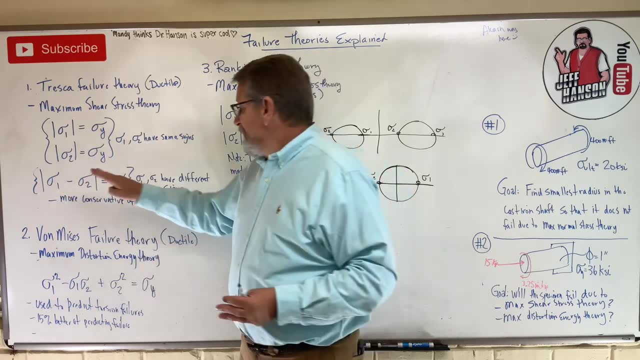 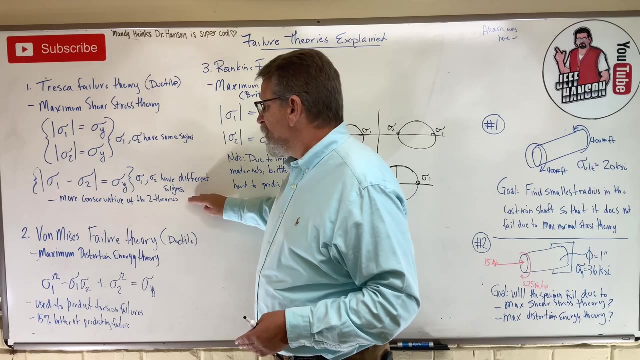 absolute value of Sigma 1 minus Sigma 2 and compare that number to Sigma yield. again, if that's bigger than Sigma yield, we got a failure. if that's smaller than Sigma yield, it's okay, all right. this is the more conservative, this one here, the maximum shear stress theory, of these two theories. okay, are these two theorems now? 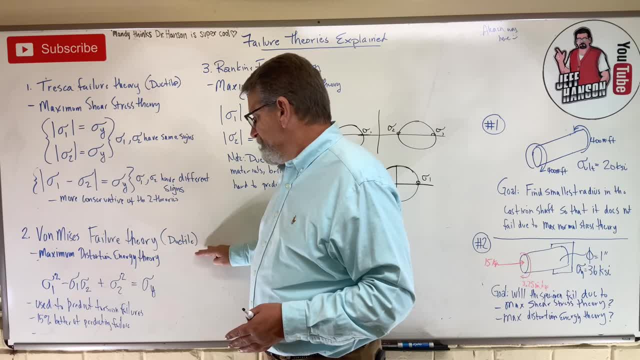 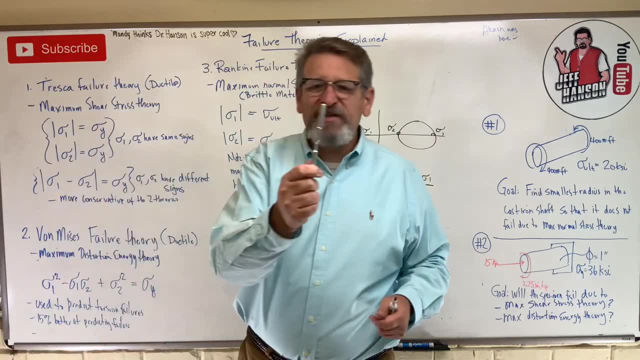 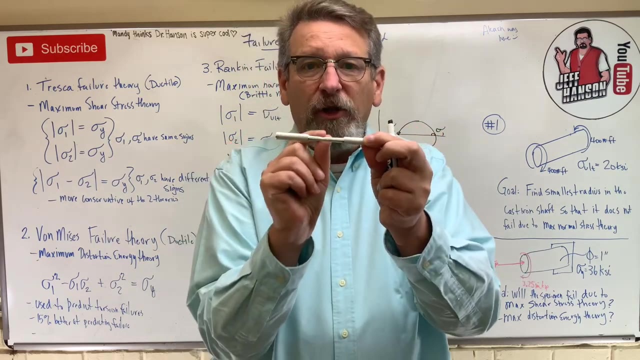 the second one is the maximum shear stress theory and the second one is the Formula one Von Mises failure theory, better known as maximum distortion energy. remember when I have a material and I have stretched it? look at that right, it's necked down there. there are little. 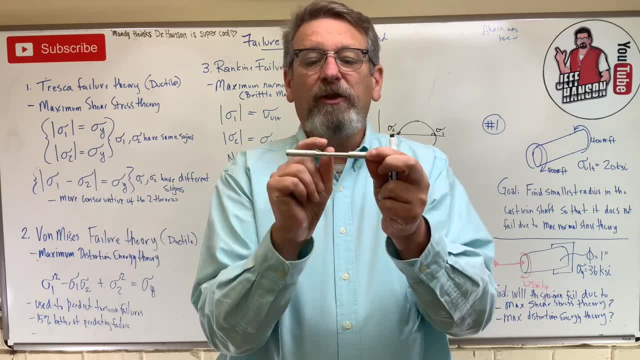 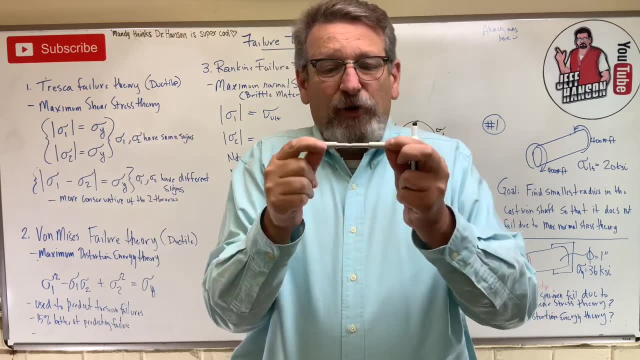 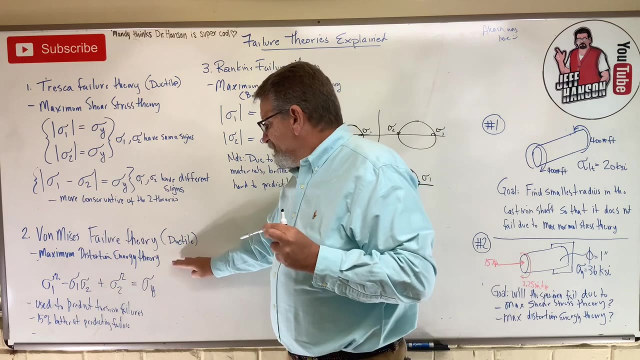 residual stresses left in the material. those molecules got stretched and now they're out of place, but they're still wanting to be back right. so there is leftover stress in this part. right, it's been hardened. There's lots of things going on there, right, That's where that distortion energy comes. 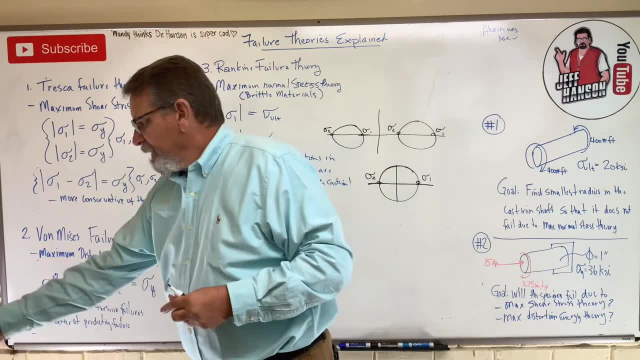 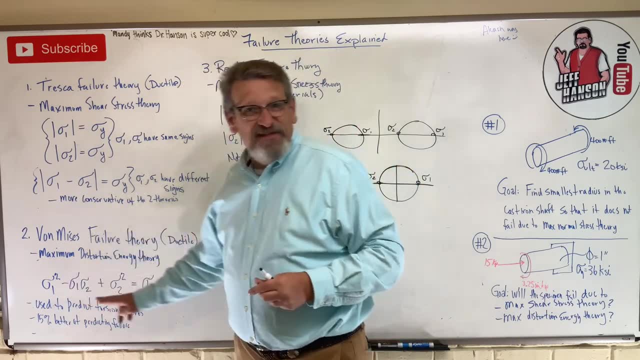 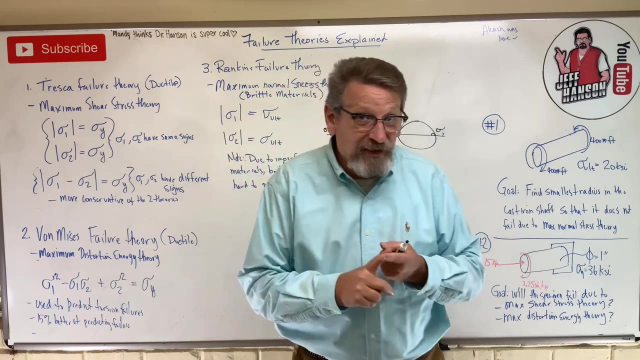 from from being stretched, from being distorted. okay, So when I use this theory here, how do you do that? Again, you have to have sigma one and sigma two. So you have to have your principal stresses. So, for all of these things, matter of fact, every one of them, the first thing you got 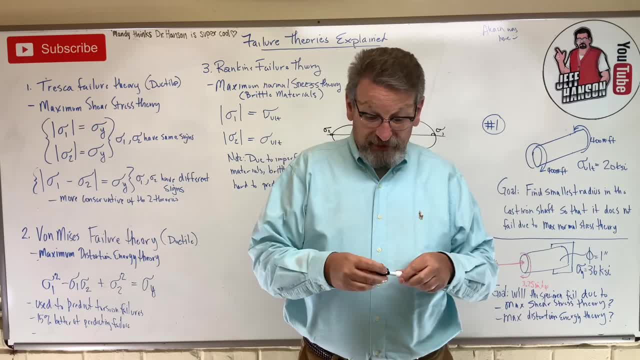 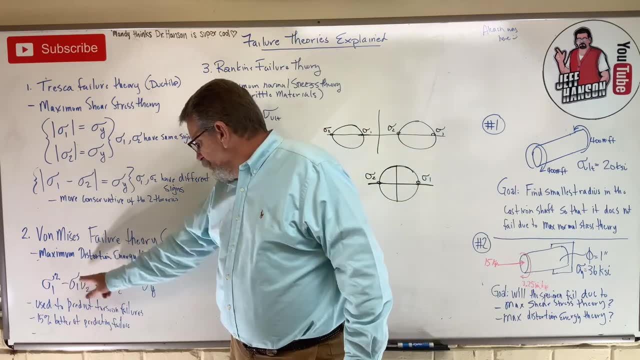 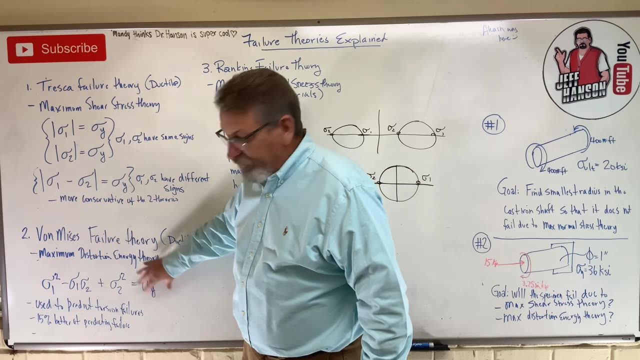 to do is do more circle and find those principal stresses right. That's one thing you got to do right off the bat. okay, But this one says: take sigma one squared minus sigma one times sigma two, and then plus sigma two squared, take that number and compare it to yield. Is that number bigger? 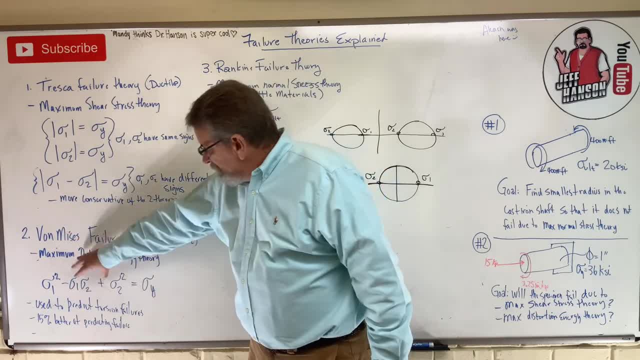 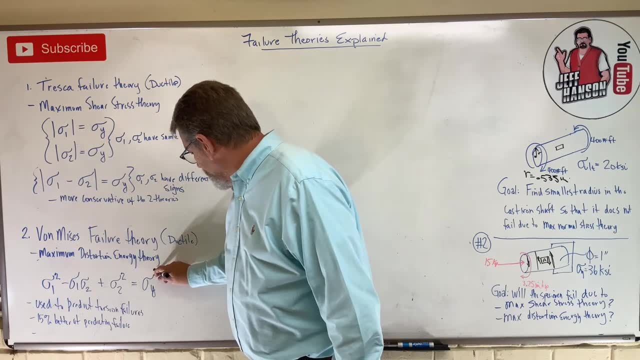 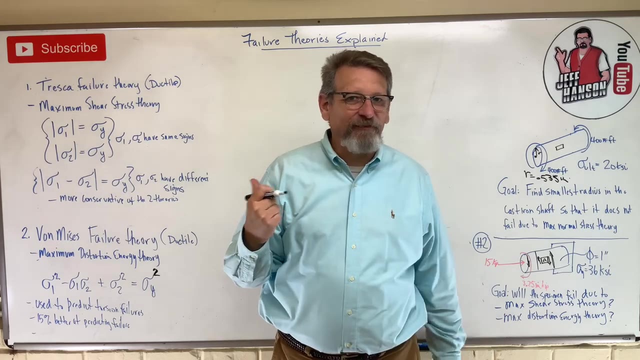 than yield, Then it failed. If that number is smaller than yield, it didn't fail. okay, Hey, Future Hanson. here There's supposed to be a squared on this sigma y, right there, Okay, Past Hanson left it off. Can you believe the guy? All right back to the video. So here I have a. 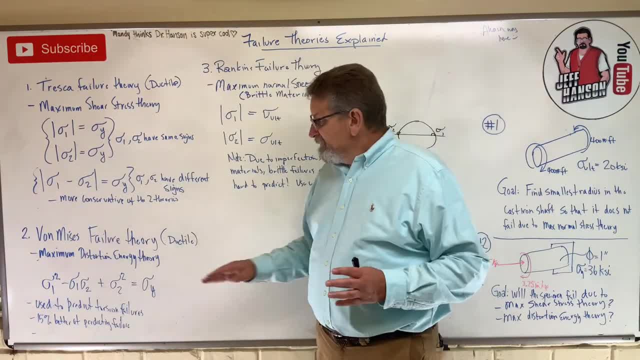 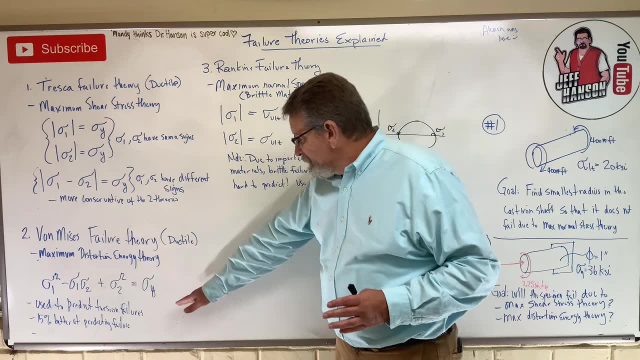 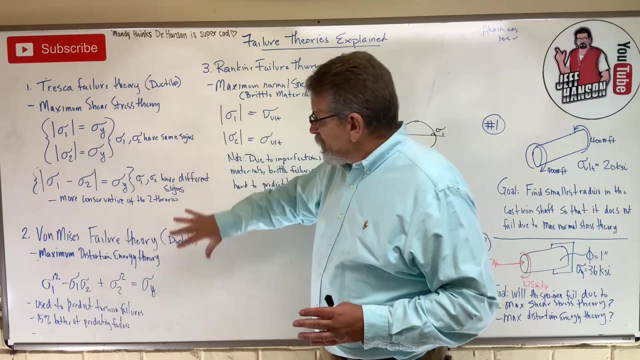 couple of notes for you. It's used to predict torsion failures. This is a really the main theory that we use for things with torsion on them. okay, Because it's about: look it says down here: it's about 15% better at predicting failure than this guy is. okay, So this is going. 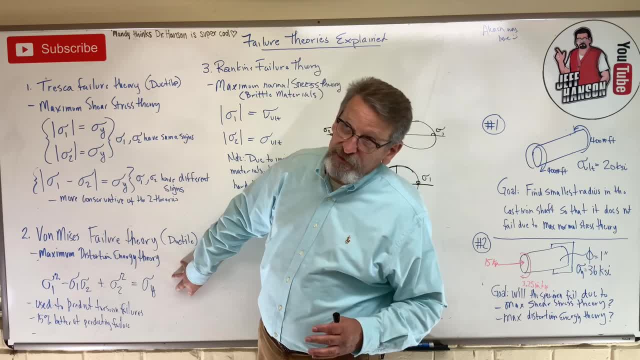 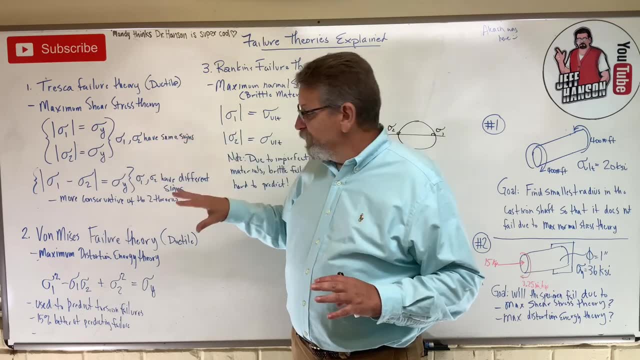 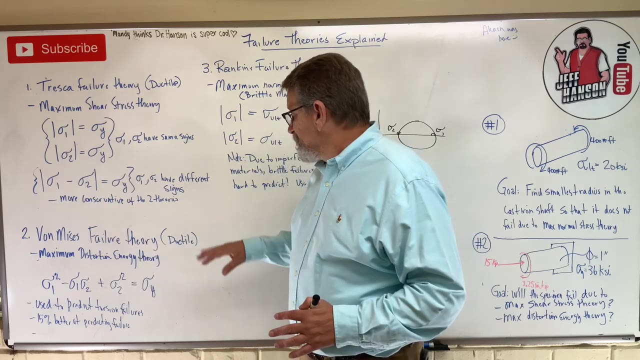 to give you a more accurate prediction of whether a material is going to fail or not- about 15% better than this guy will. okay, Like I said, that's more conservative. If you want really a more accurate, you need to come down here and use von Mises, okay, So von Mises is just another. 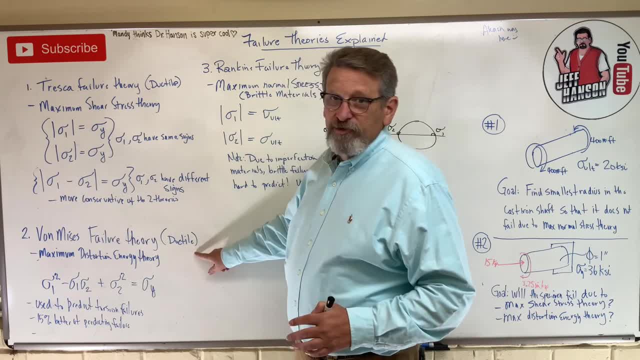 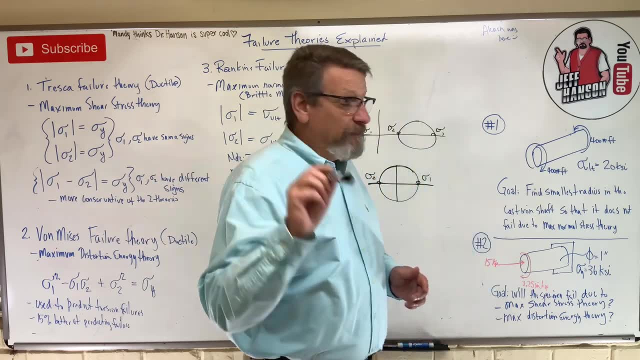 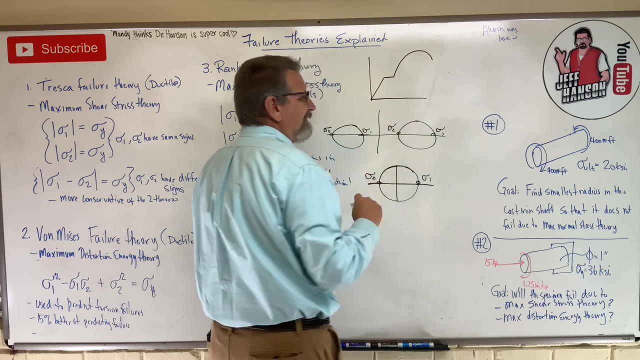 theory. But again, these two theorems here are for ductile materials. And notice, we use yield. We're comparing to yield for ductile. Now, if we think about, if we think about brittle materials, right, Ductile materials- remember our stress-strain diagram? looked like that, didn't it? 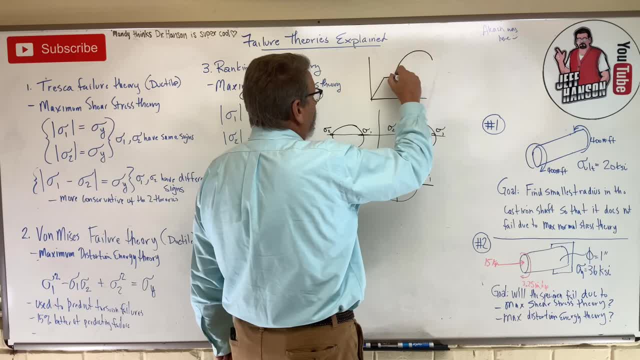 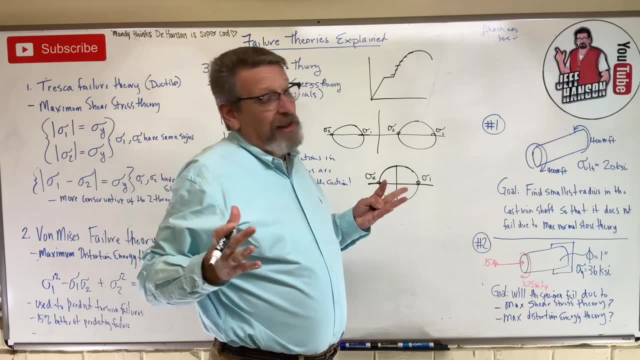 Okay. So on ductile material, this, all, all of this up here, is yielding right, Yield, yield, yield. So a ductile material stretches and it's telling you: I don't like this, Something's going on. You know, it gives you a warning that there's going to be a failure, Whereas brittle materials 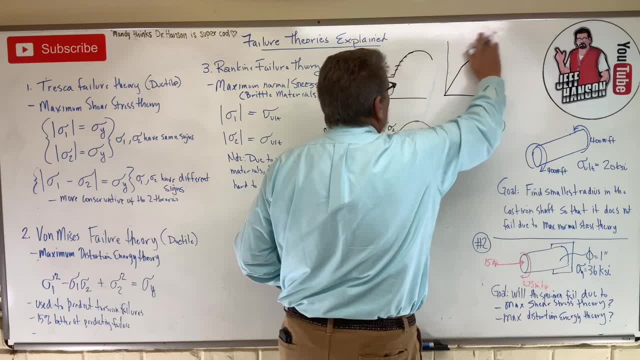 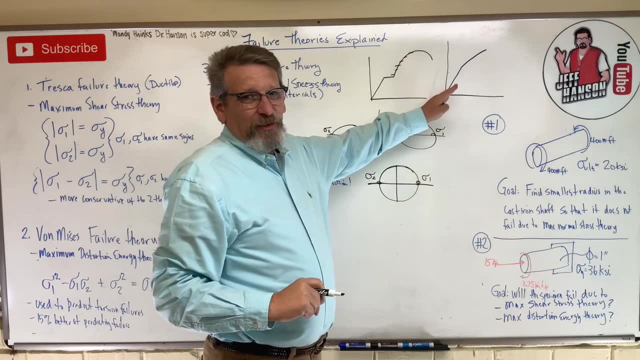 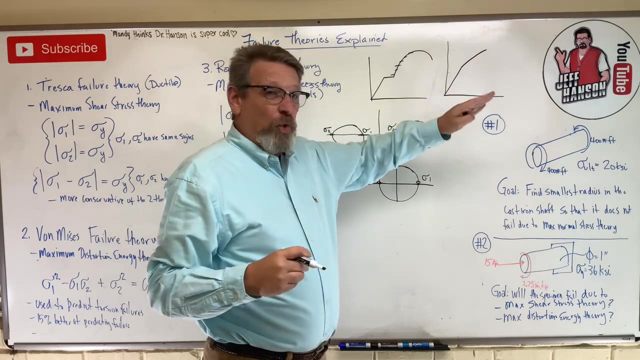 right, Do something like this, okay. Brittle materials: do something like that- okay. Now on a brittle material. the thing we don't like about brittle materials is, all of a sudden they just fail, okay, And so they don't give you much warning that they're going to fail. 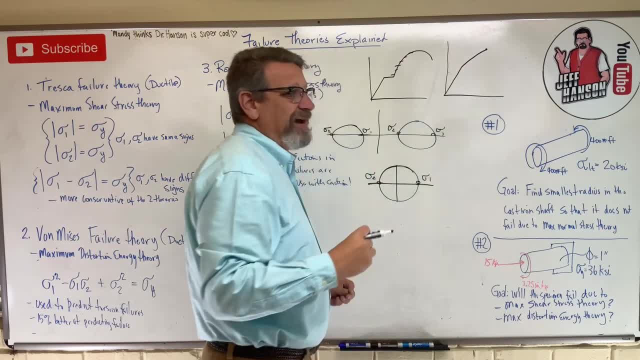 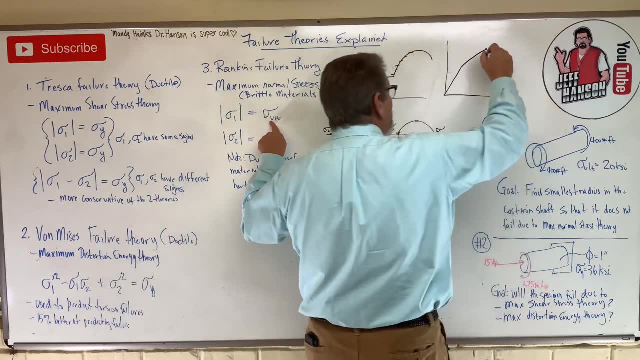 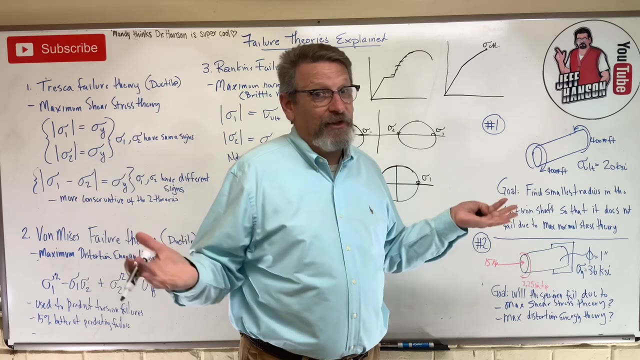 Okay, So on a brittle material we don't really have a lot of yield stress warning. So what do we do on the brittle materials? We look at this point up here, which is sigma ultimate right, Because at that point it just breaks. So, brittle material, a fracture is the failure. 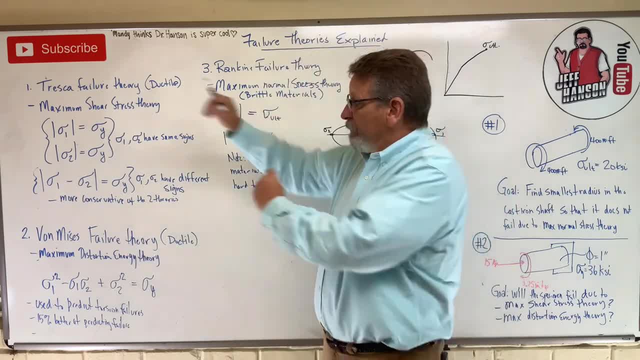 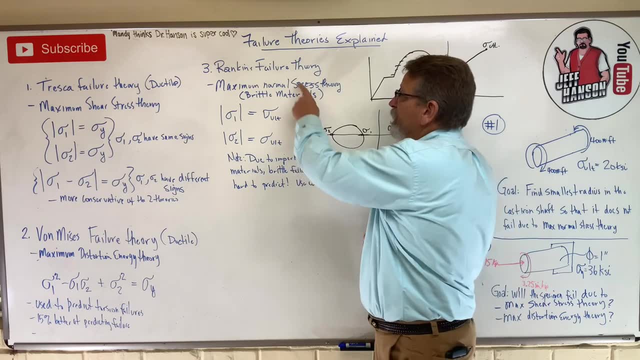 right, We don't want that to happen. Okay, So in ductile materials we're looking for yielding, In brittle materials we're looking for ultimate And again, it's pretty much the same thing. This one Rankine failure theory is called the maximum normal stress theory. 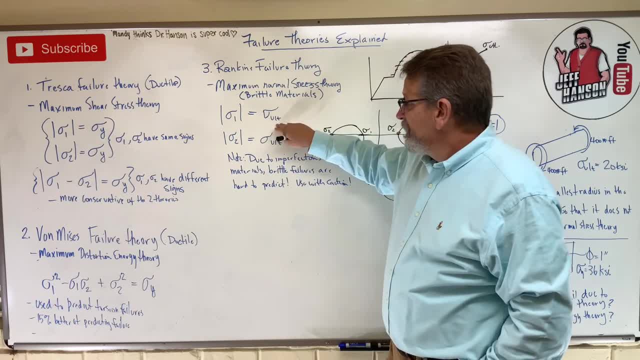 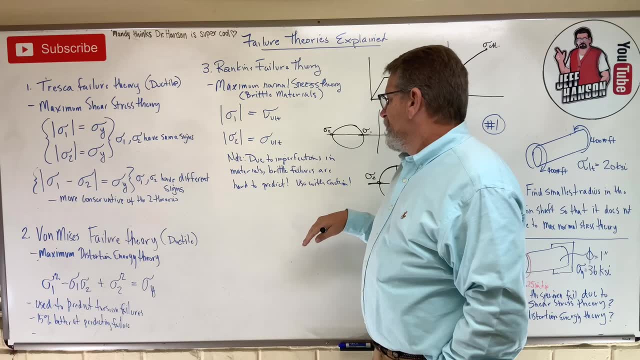 Again used for brittle materials, And you can tell that because of the ultimate okay And you just use sigma one, you know if you're on that side, sigma two if you're on this side. whichever one of these two is bigger, whichever one's bigger of the principal stresses. 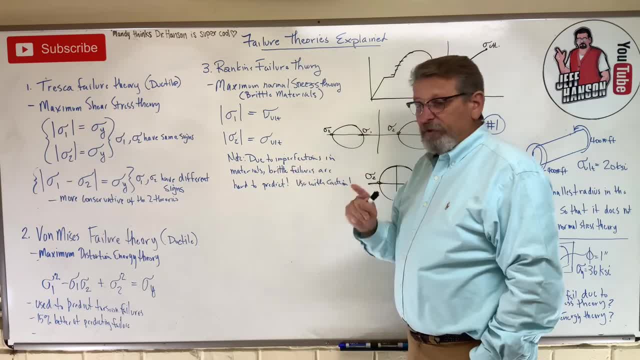 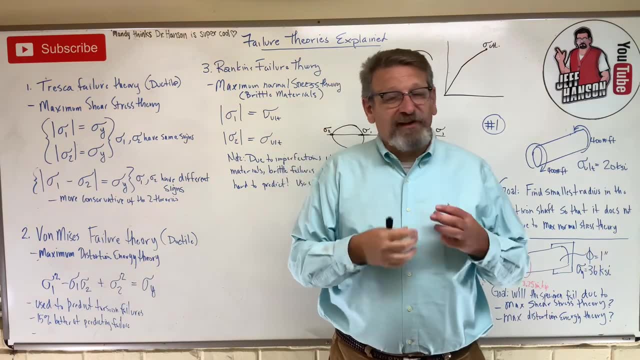 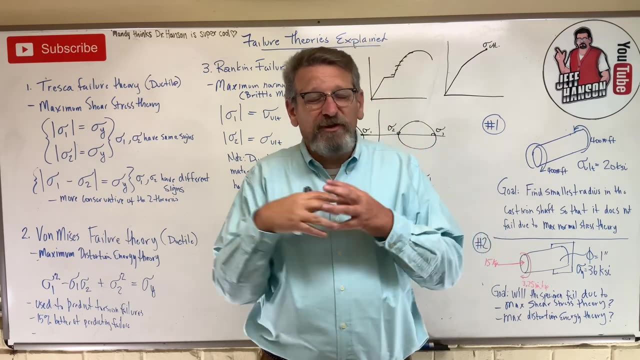 And again, due to imperfections in materials. brittle failures are hard to predict. Use with caution, okay, Because in brittle materials like cast iron, glass, right, There's imperfections in the material, There's imperfections in the crystalline structure, There's a lot of things. 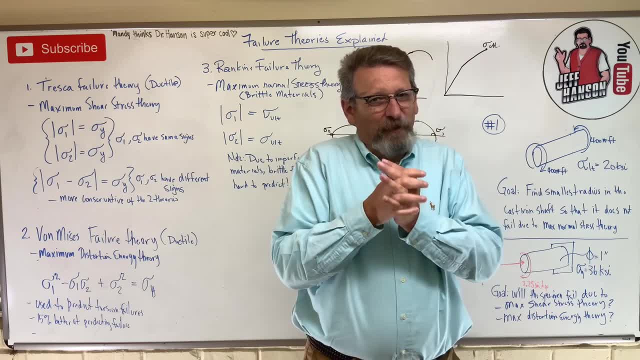 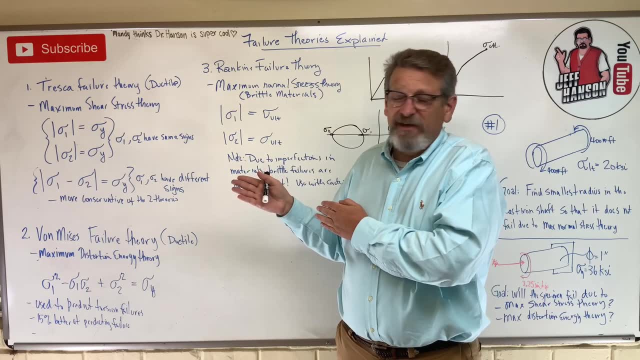 that in the casting there's a lot of things that couldn't be just perfect, And these numbers here are, assuming, kind of as close to a perfect material as you can get. So you know if you're going to use these numbers and say, okay, I'm going to design. 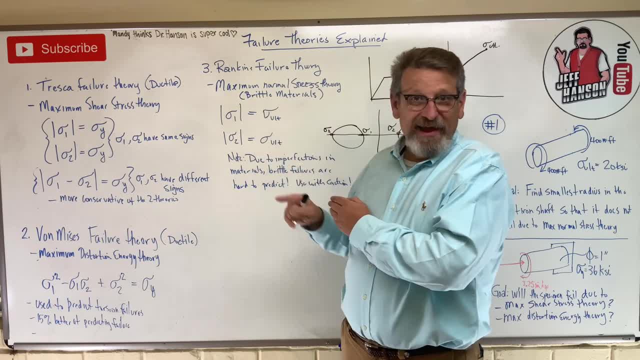 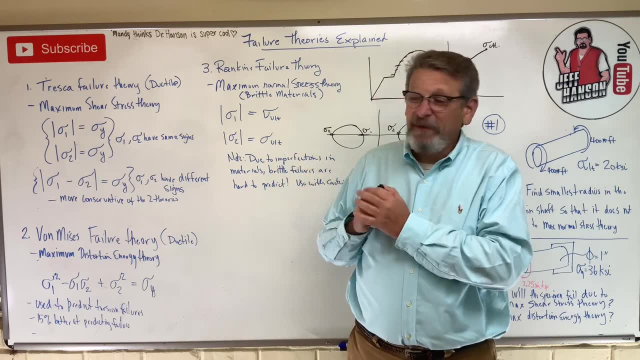 something for that number right there which is right at ultimate. it's probably dangerous, right, Because you're probably going to have some imperfections, that's not going to be quite that strong. So what do we do with those? Hey, you remember, we use a factor of safety, don't we? 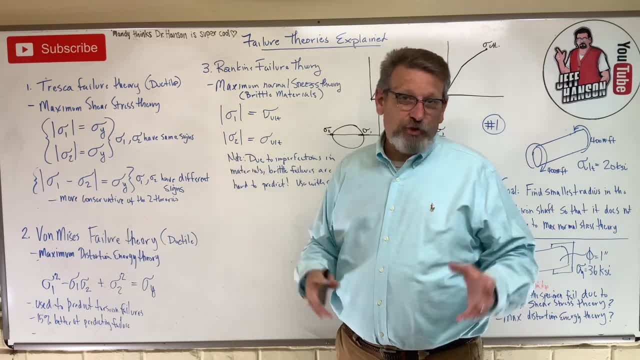 We'd want to put a factor of safety with these to make sure that they don't fail, Because we don't want to design something that's going to be right at yield. We don't want to design something that's going to be right at yield. We don't want to design something that's going to be right at yield. 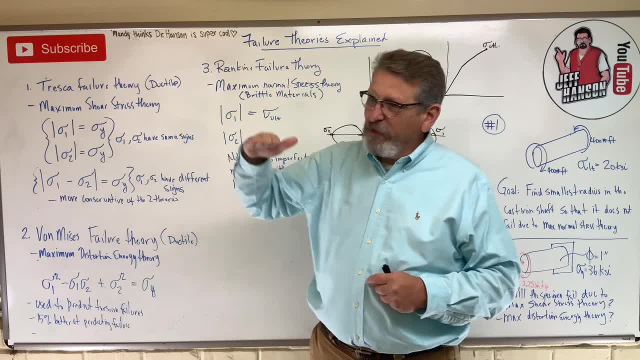 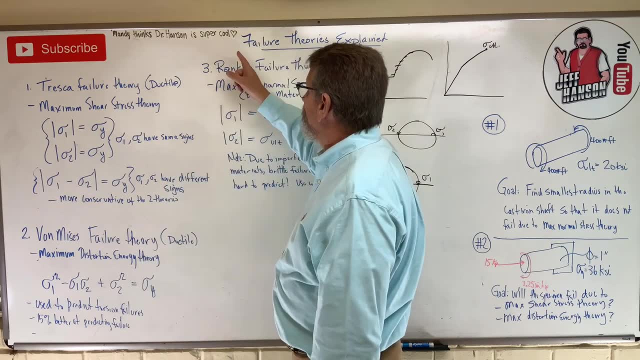 We want to design something that's going to be right at ultimate- okay. We want to factor safety so that we can back that up, okay, All right, I see that my students have been in here and Mandy thinks that I'm super cool, So you know. thanks a lot, Mandy, Okay. 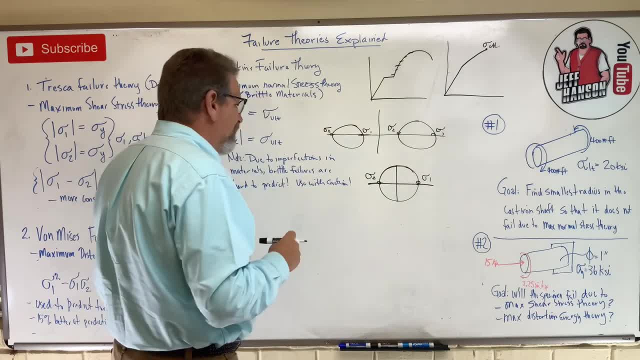 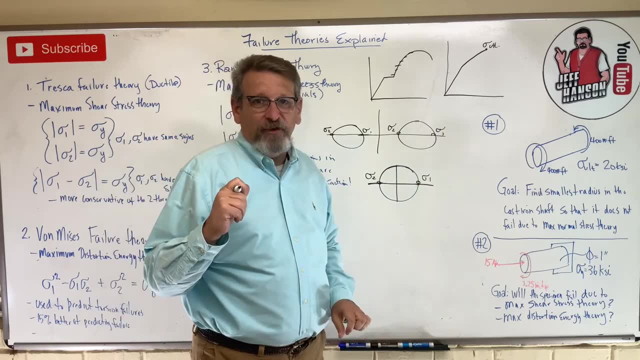 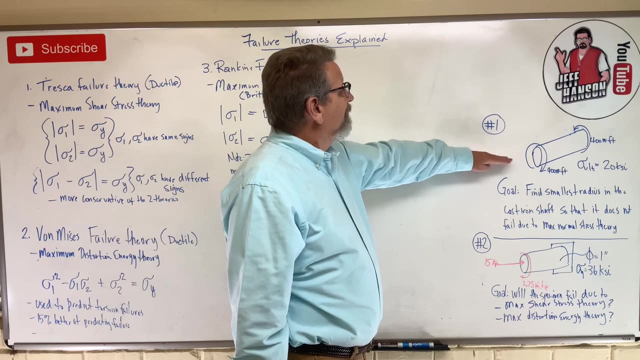 All right. So let's see if we can work some problems using these theories over here of failure and see if we can predict whether these are going to fail or not. All right, Let's try number one. here We have a piece of cast iron. It's cast iron. What does 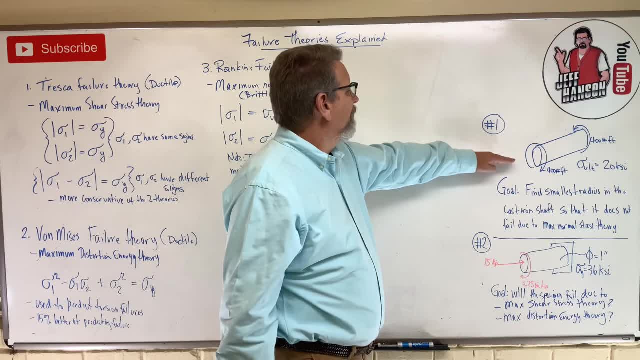 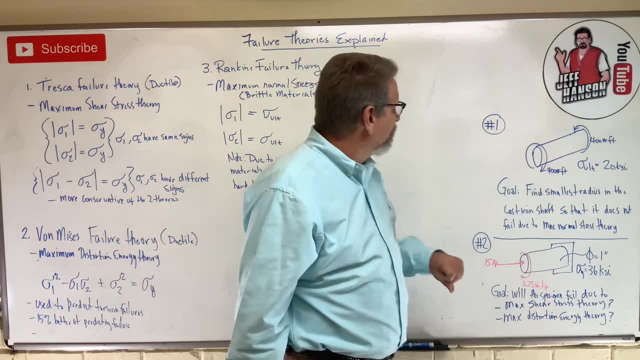 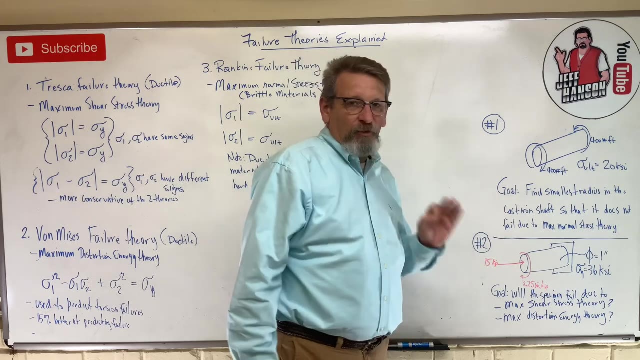 that mean That's brittle. Yeah, it's brittle. okay, They give us. the ultimate stress is 20. KSI has 400 pound feet of torque on it. okay, Find the smallest radius in the cast iron shaft that it does not fail due to the maximum normal stress theory, which is this one. Hey, 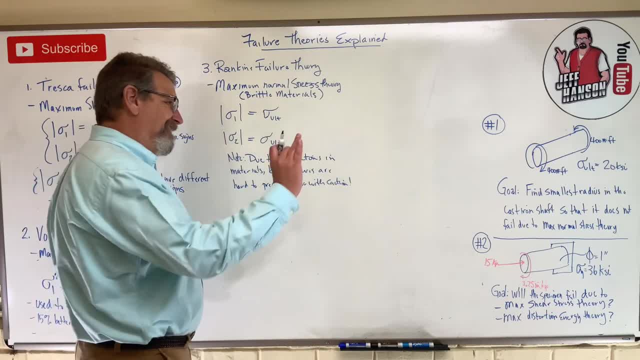 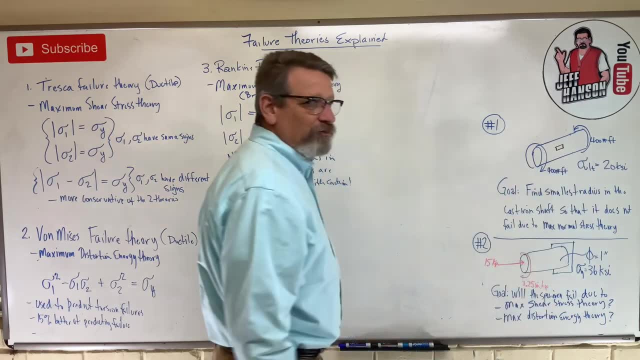 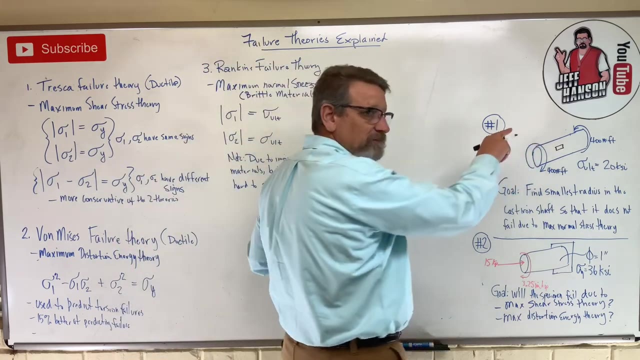 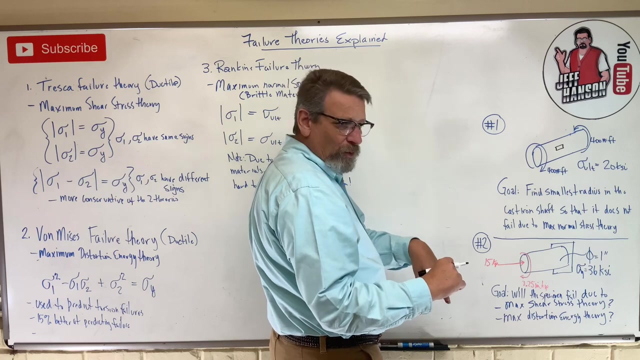 that's the one for brittle materials, cast iron. Hey, all right, Okay. So if you're a little piece of material right there, right, A little stress element, if you will, what are you feeling? Okay, Well, is there anything stretching you P over A? No, Anything bending you MC over I? No. 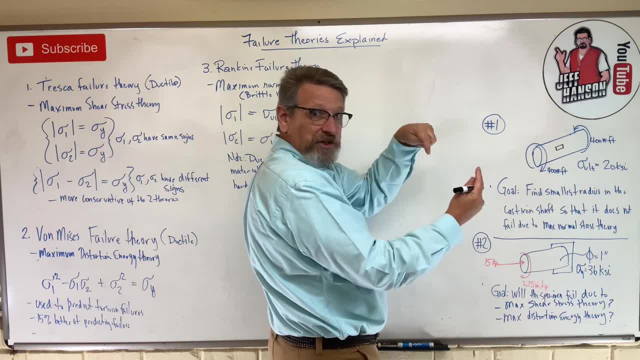 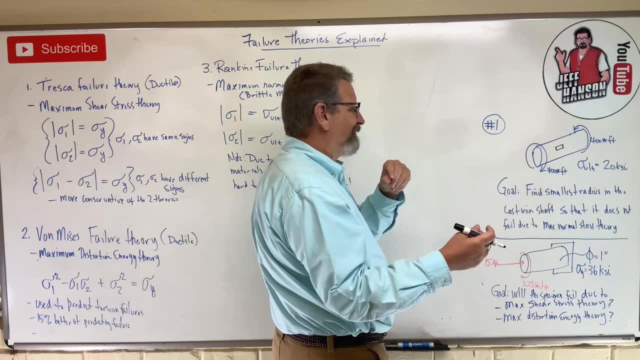 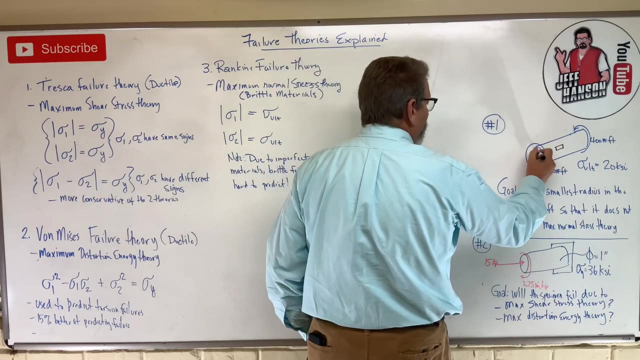 Is there any shear forces? Transverse shear: No, Is there any TC over J? Torsion shear? Yes, there is right. Okay, So here we go Now. we don't know the radius. okay, So the radius, let's just call him R. okay, So tau, right, Tau. 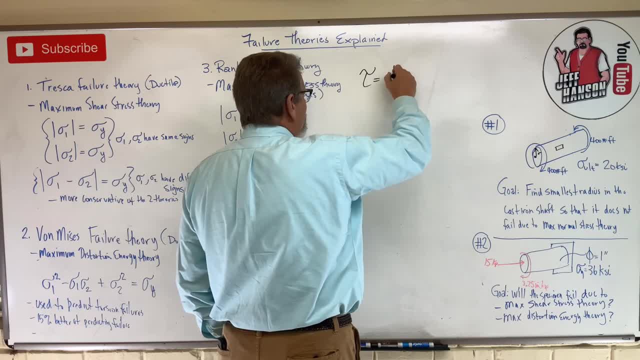 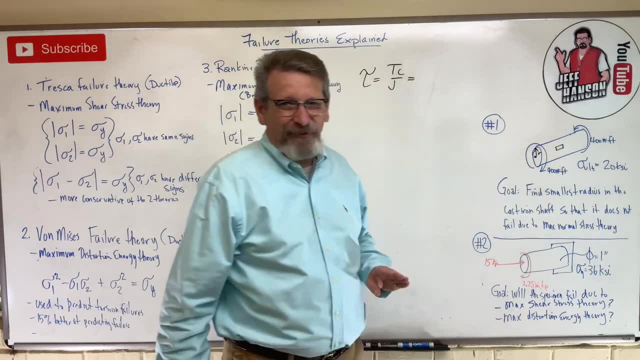 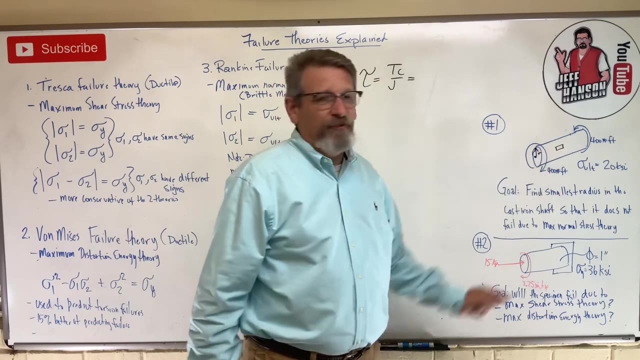 is equal to TC over J. okay, So T, what is T Now? Johnny Weeks tells us. is he in the house? Johnny Weeks tells us would say: yo, that's got 800 pound feet of torque on it, 400 there and 400 there. 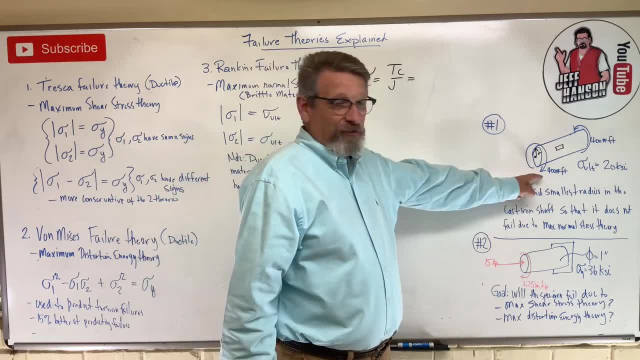 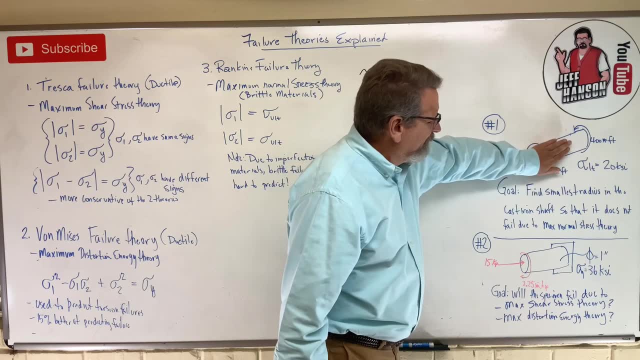 No, Johnny Weeks tells us, no, It's only got 400, right? Remember this 400 causes that 400 over there. Remember, if I section it in half, if I just look at half of it, how much torque is on? 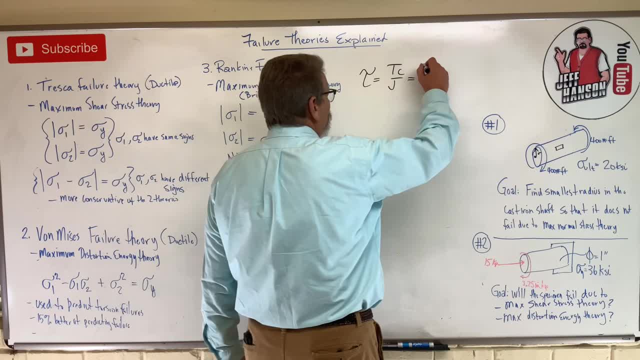 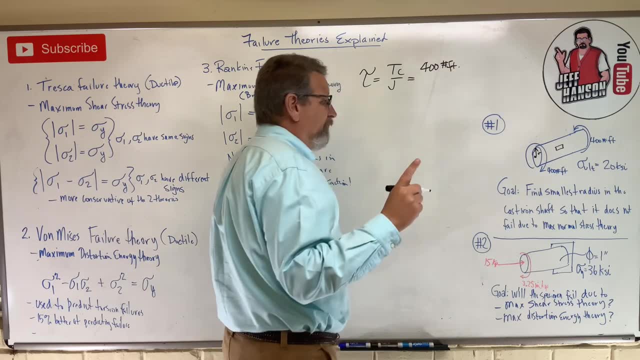 there Only 400, okay, So here we go. Torque, 400 pound feet. Now got to be careful, because I'm thinking this radius is going to be in inches and that's in feet. Let's get rid of that, feet up. 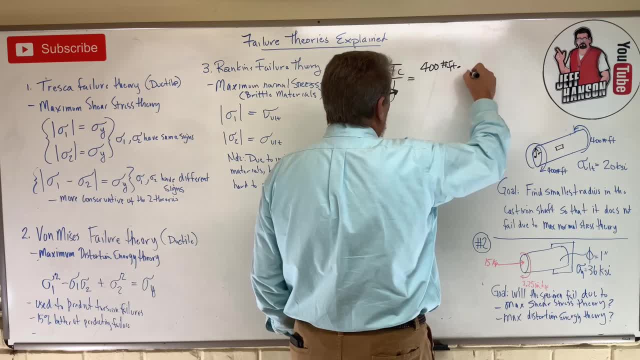 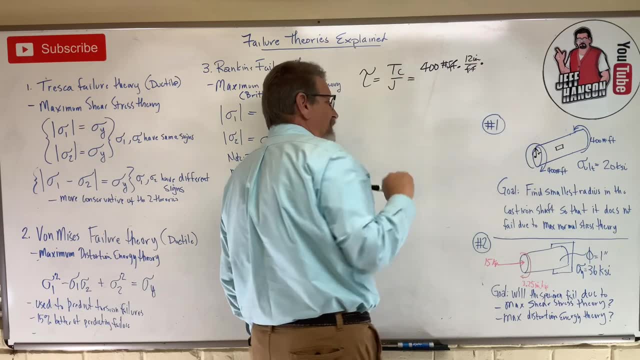 there, okay. So let's multiply that by what Let's get. feet on the bottom is 12 inches on the top. That'll get rid of that. guy Times C. What is C? The distance from the neutral axis to the outside. 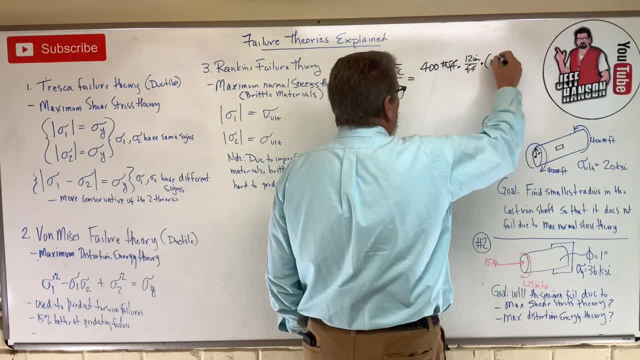 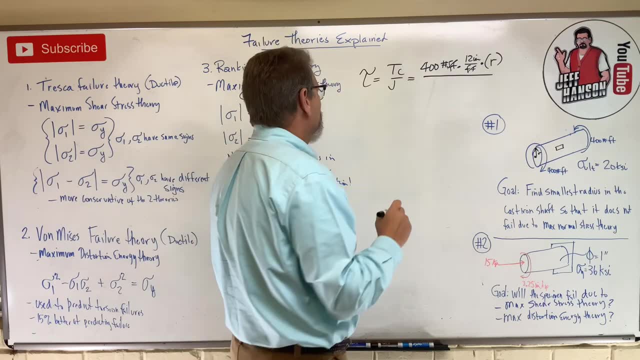 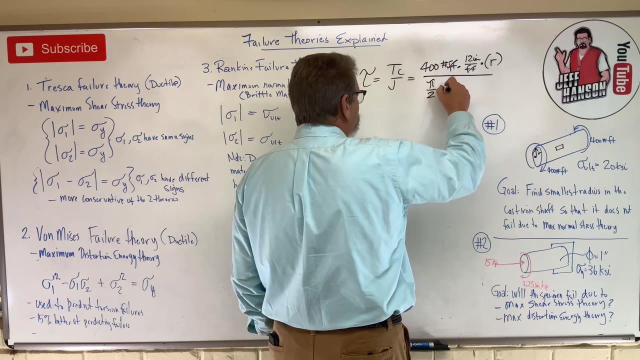 of the part. okay, In this case it would just be R divided by J. What's J for a solid round shaft? That would be pi over 2 R to the 4th right. All right, and so what can we do with that? 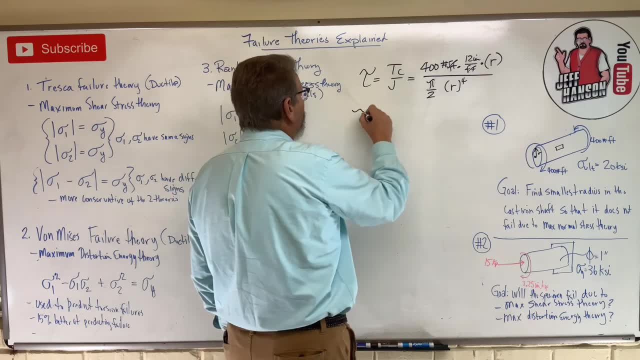 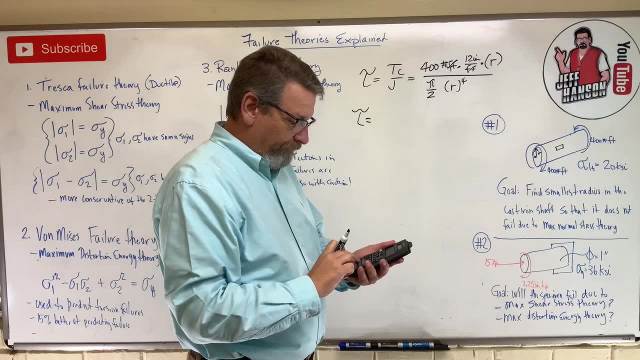 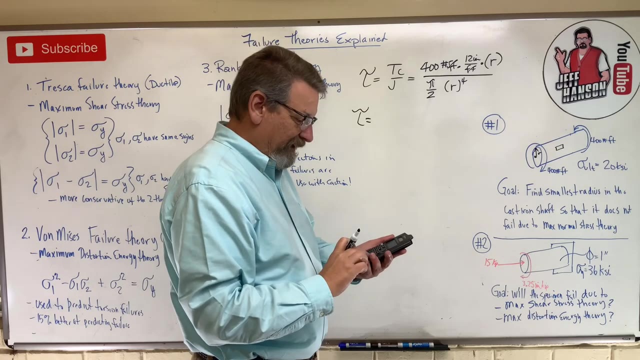 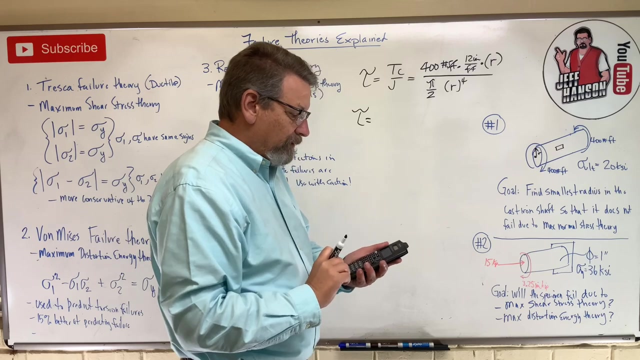 Well, here's what we can do with that. Tau is equal to- let's do a little math here. Let's math this up: 400 times 12, 400 times 12 equals, and then divided by pi over 2.. Pi divided by 2 parentheses: 30, 55.77. 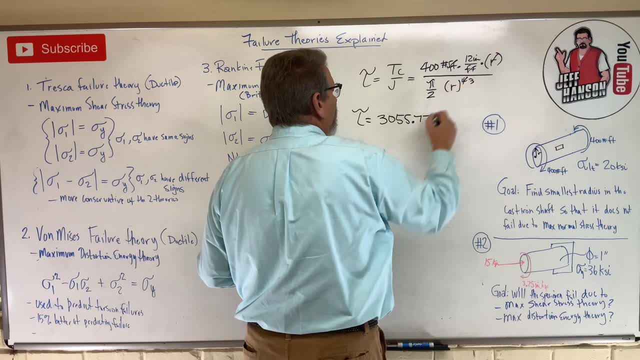 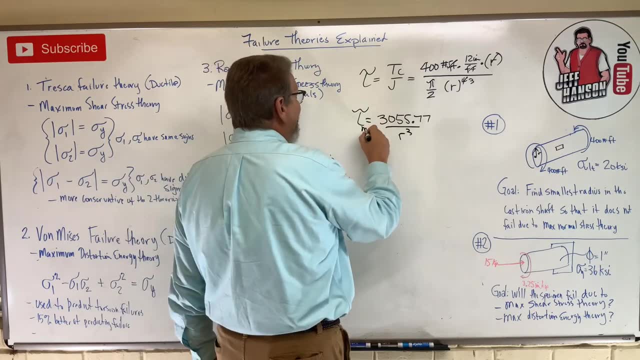 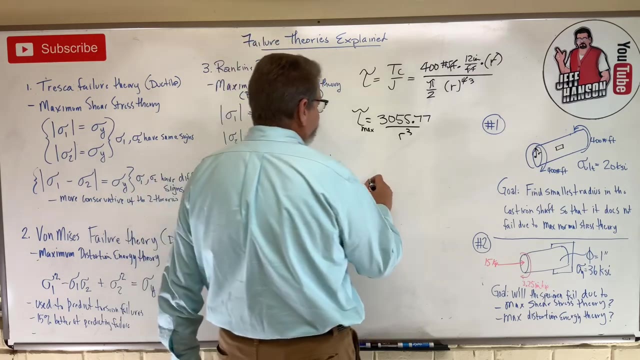 And then divided by what One of those R's is going to go away, Divided by R cubed, Do you agree? Okay, so that's tau max. That's the biggest shear on that shaft, is tau max? okay? Now, if we were to draw more circle? okay, we already said there was no sigma stress. 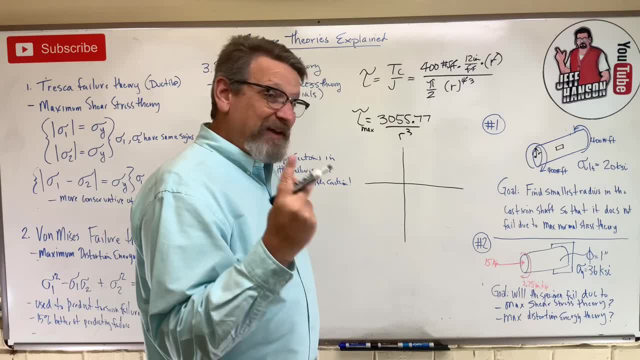 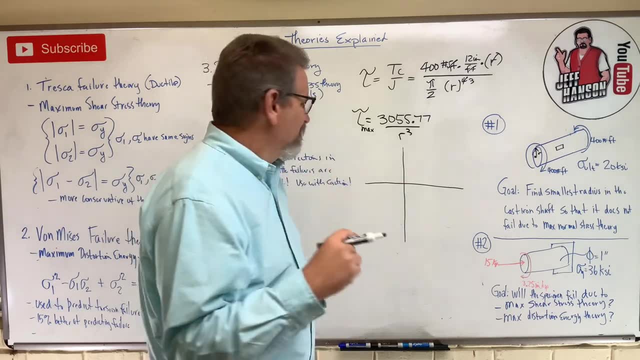 There was no MC over I, There was no P over A. which means what That? sigma at zero for that guy. all it has is shear stress on it, right? So all it has is a number here and a number there. 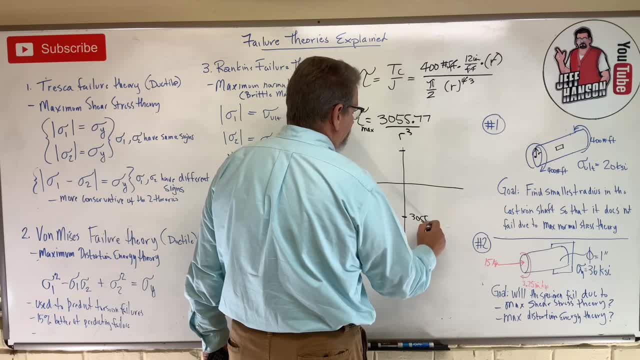 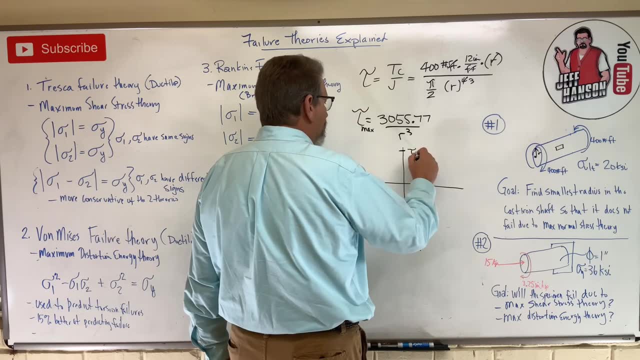 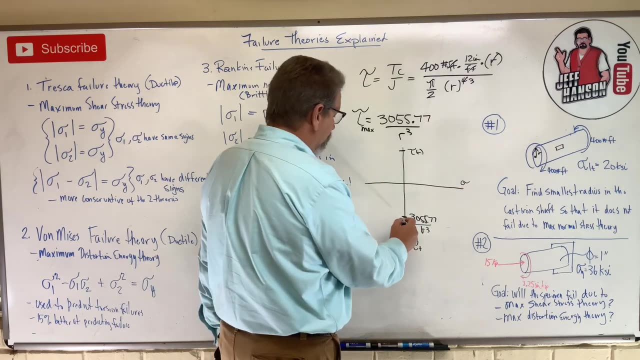 right, Which is that number is 3055.77 over R cubed right. Remember, this is tau positive down here. This is tau negative up there. This is sigma right. Can I draw a circle out of that? Well, yeah, It goes like this: 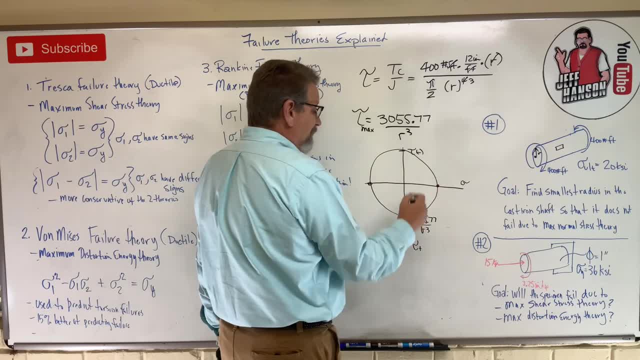 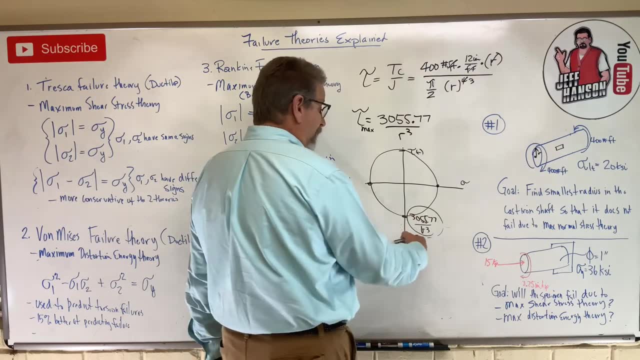 Kind of circular. What does that mean? If tau is that number, what does that mean? sigma 1 is Sigma 1 is that's a radius right. That means sigma 1 is that number. So sigma 1 is equal to. 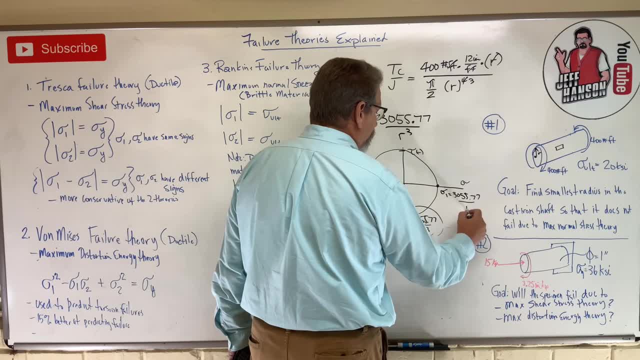 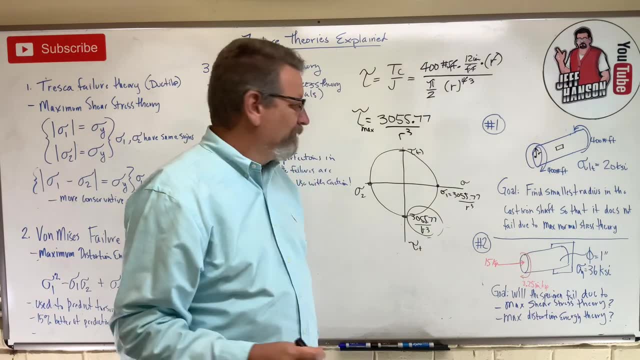 sigma 1 is equal to 3055.77 over R cubed. And guess what? So is sigma 2, right? They're the exact same thing. So if we want to find out what it can take, then we should just set this: 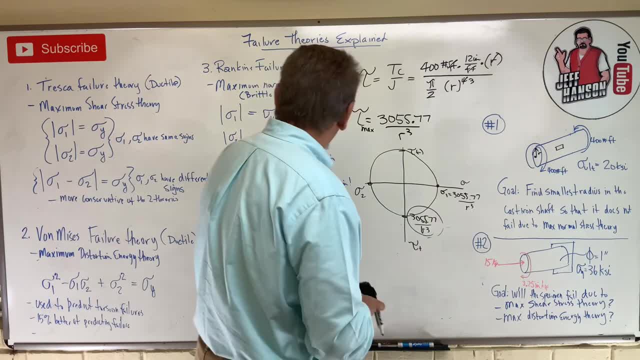 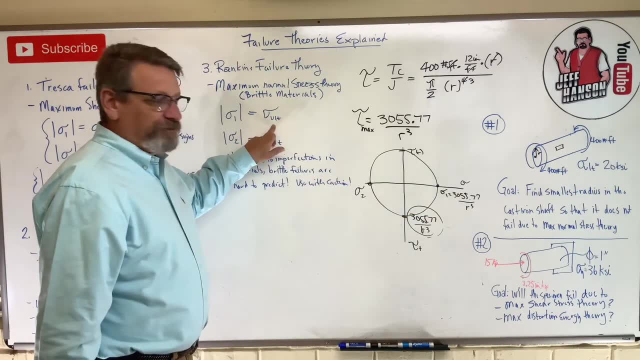 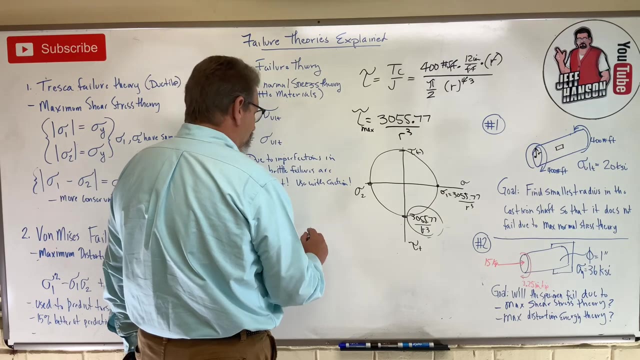 equal to what right? What does this say? do? It says: take sigma 1, which is that- and set it equal to the ultimate stress. okay, The ultimate stress is 20 KSI. okay, So this is going to be 20, oh, don't fall for that little. 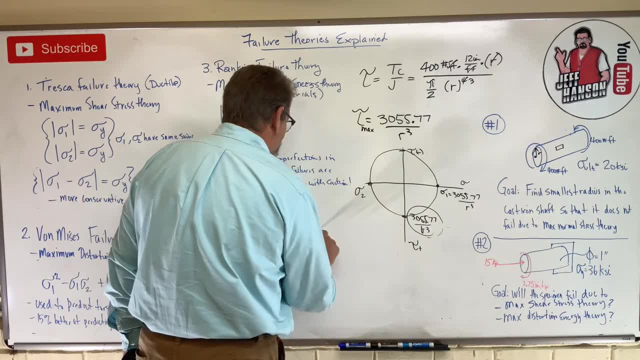 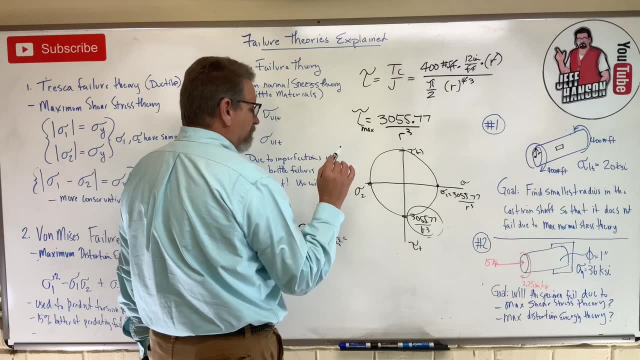 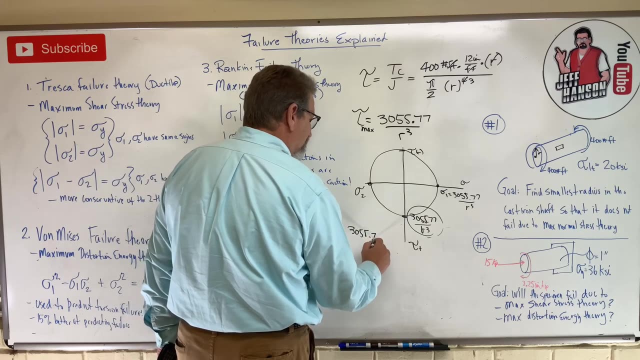 trick KSI, that's kips right. 20,000 pounds over inches squared is equal to T. which is what? No, it's equal to T, It's equal to sigma 1, it's equal to that right. 3055.77 over R cubed. 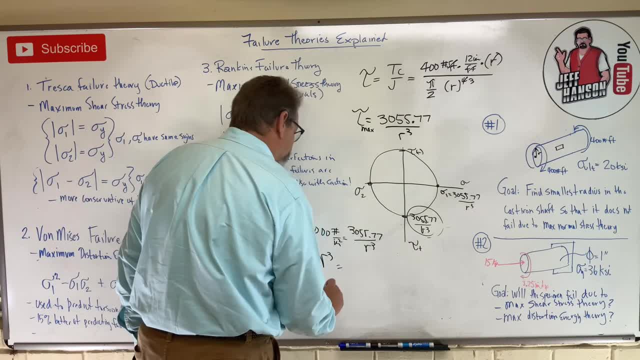 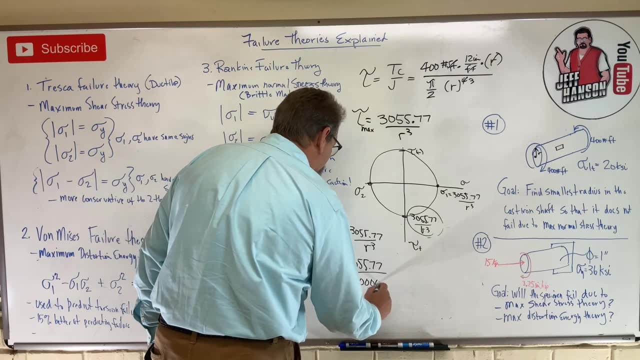 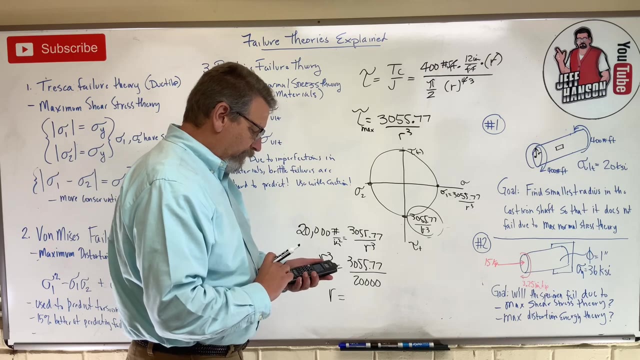 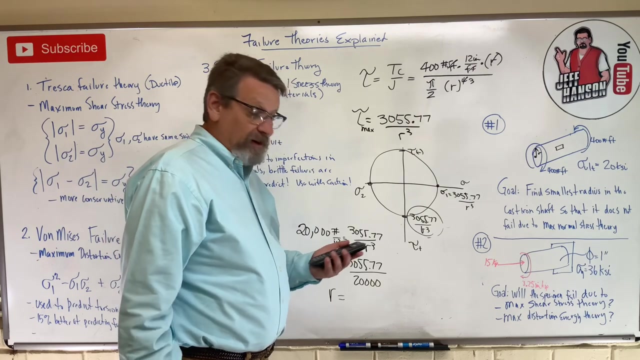 so R cubed equals 3055.77 divided by 20,000.. So R is equal to: here we go. divided by 20,000 equals. and then second cube root. oh lordy, All right, I forgot how to put that in my calculator. 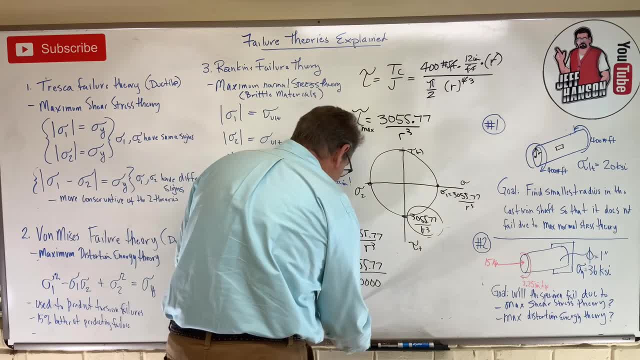 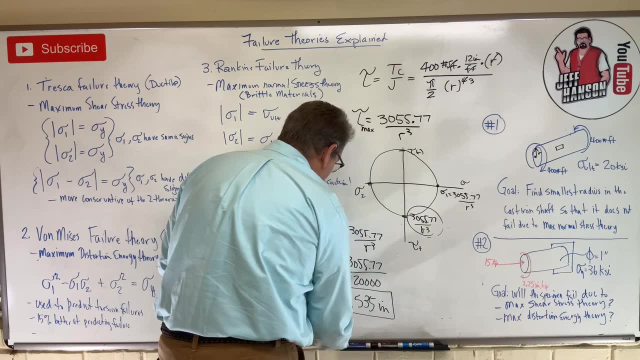 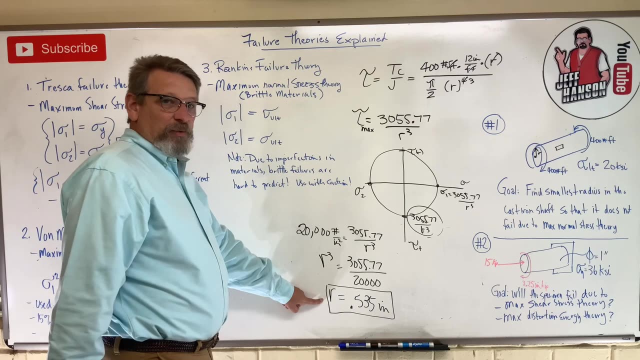 but I figured it out, And R is equal to point 535 inches. okay, There you go. So for that not to fail, for it not to fail, it needs to be at least 0.535 inches or bigger, right, It can be bigger than that. 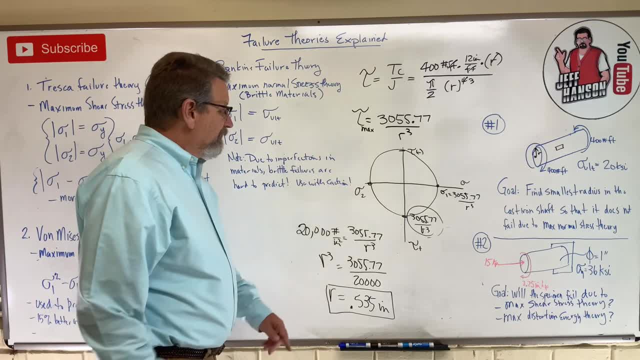 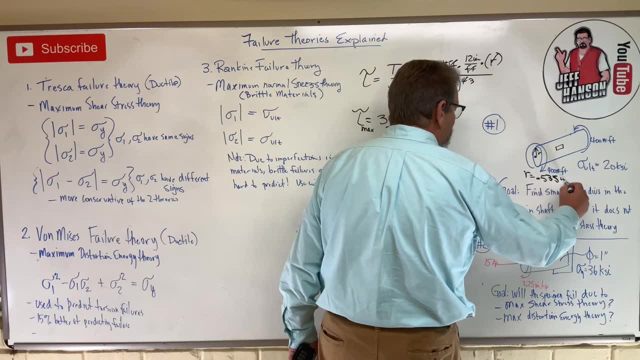 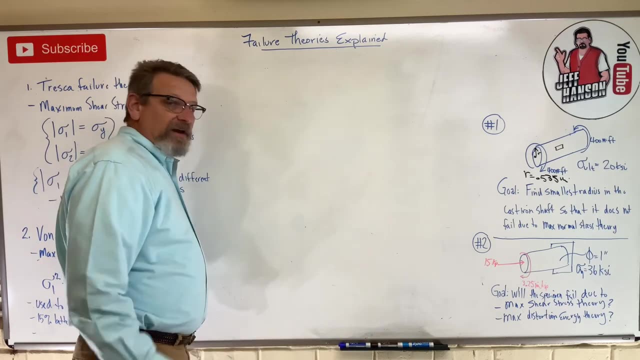 but that's as small as it could be right there. okay, So that's the answer to number one. Number one: R equals 0.535 inches. Well, that's not too bad. Let's see if we can do. number two. Okay, here we go. Number two says: 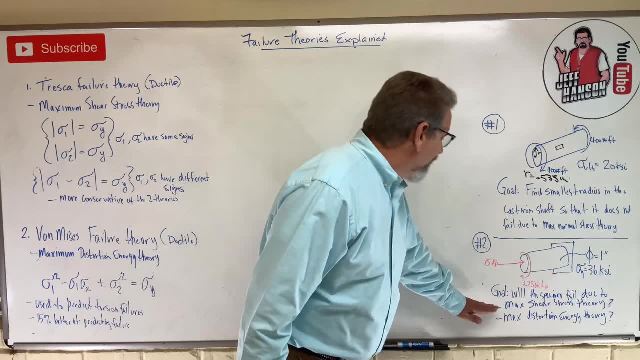 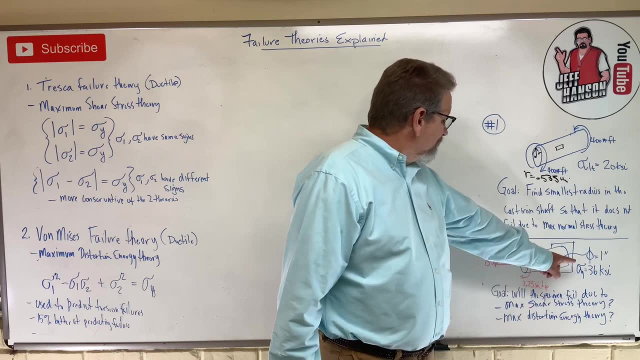 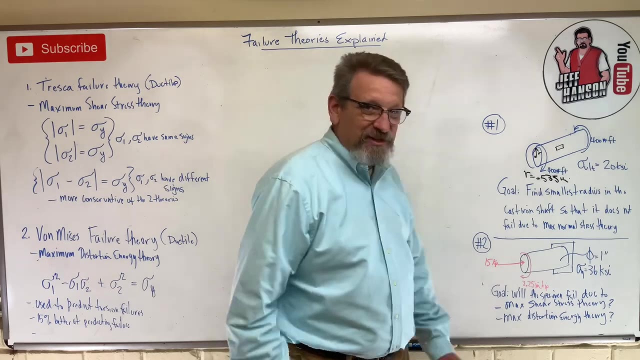 this: Will the specimen fail due to maximum shear stress theory? Huh, Now it's A36 steel. okay, The steel specimen. And so guess what We're talking about a ductile material here. So will it fail due to maximum shear stress theory? I erased the brittle theory There. that's this guy. 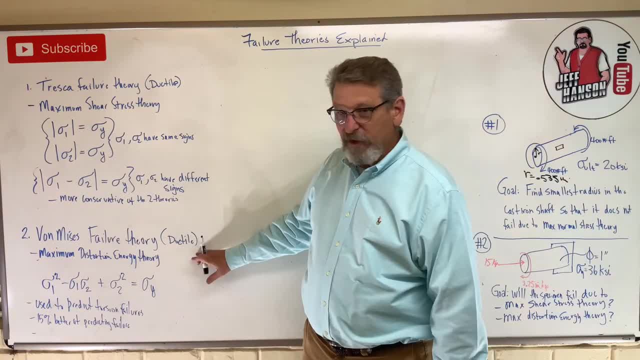 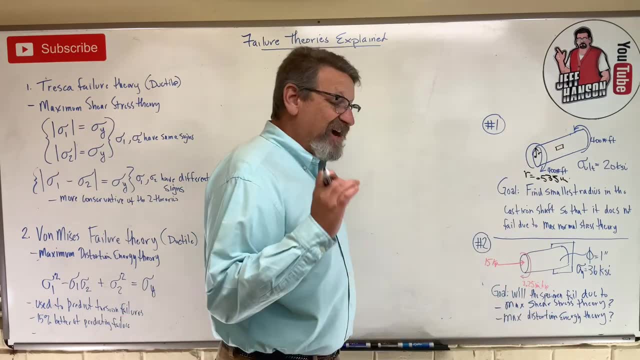 It says: will it fail due to that theory? right? So we're going to test it using this guy, then we'll test it using that guy. We'll see if they give us the same results or not. okay, So this is kind of a combined loading problem to start off with. Look, I got a specimen here. 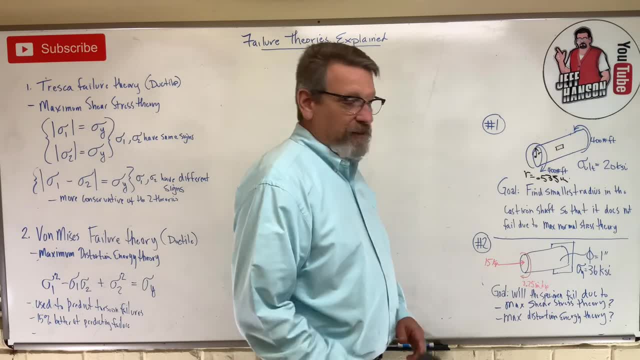 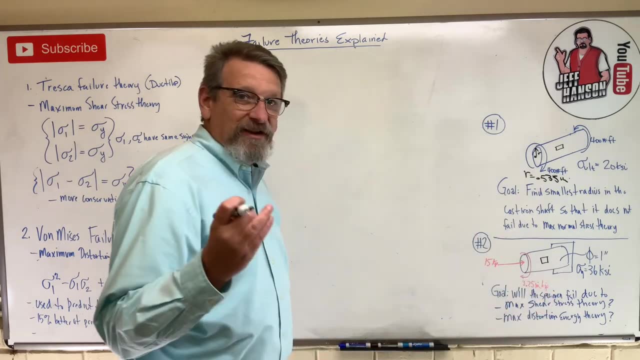 that has torsion on it and it has a load on it, a compressive load Again. if I was that little stress element- because I like to think of that little stress element, because that's what I'm going to use my Moore's circle to transform right. 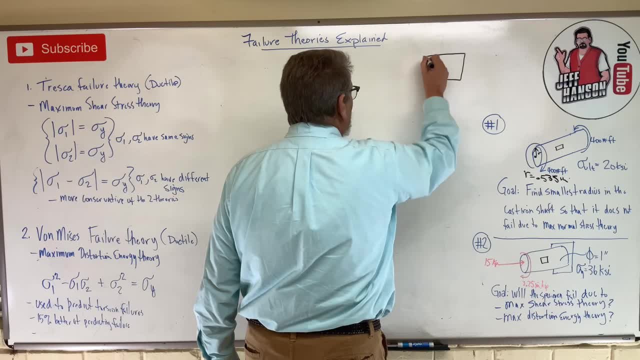 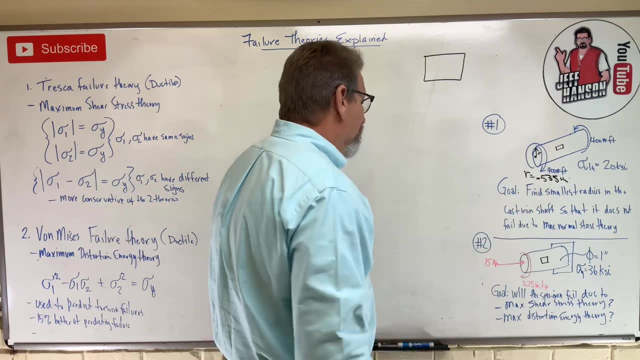 So if I'm that little stress element here I am, what am I feeling? okay, I think I'm feeling a compression. I think I'm feeling a P over A. don't y'all All right. so what do we got here. 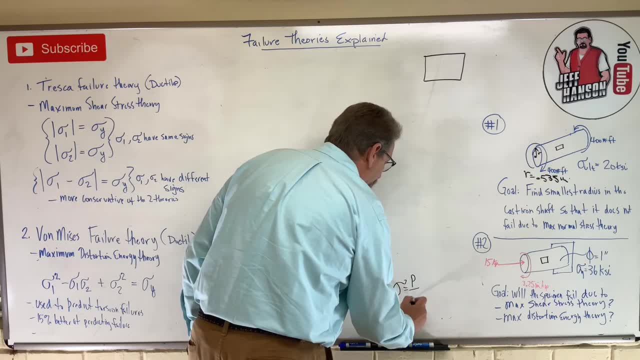 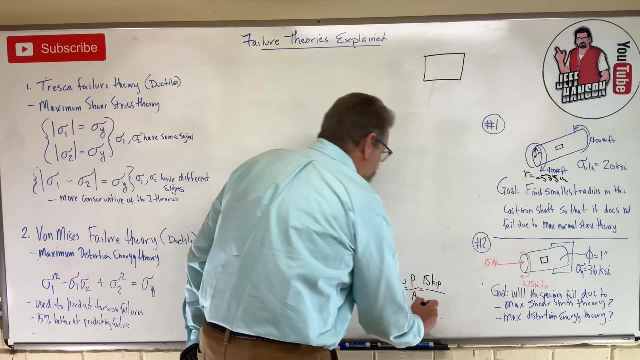 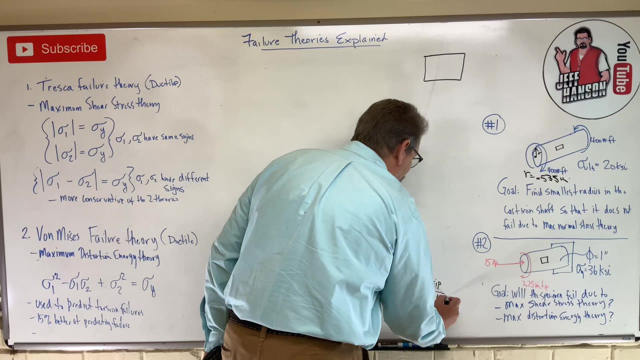 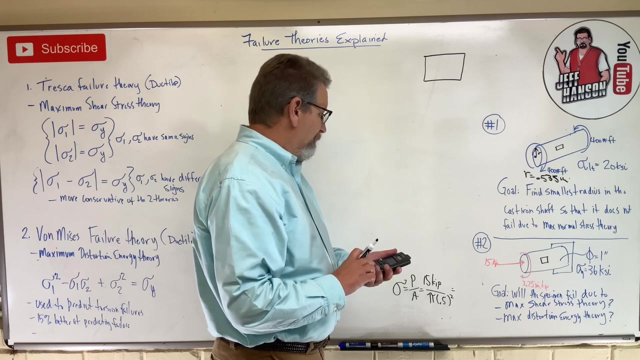 So sigma equals P over A. equals what 15 kips divided by A, which is pi times R squared, and R is it's an inch diameter, so 0.5.. 0.5 squared, what does that equal to 15 divided by? 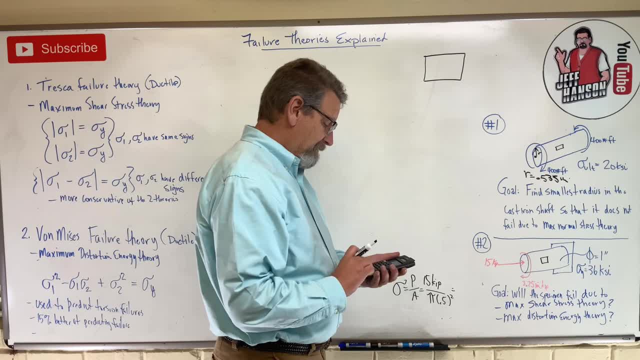 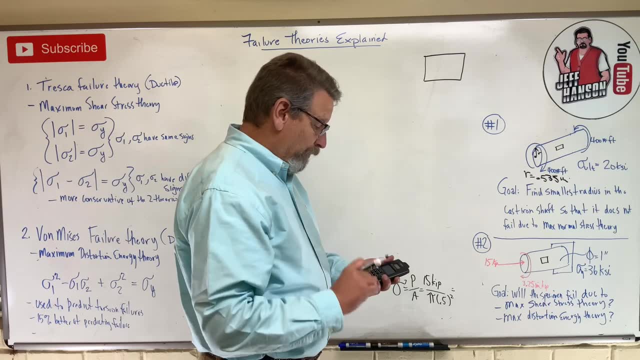 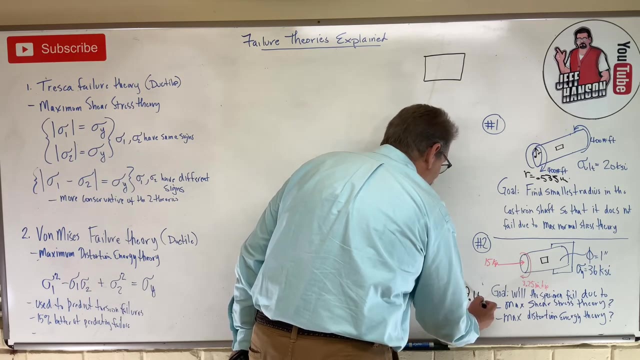 pi equals divided by 0.5 squared equals 19.01, 19.1, and that's going to be what. That's KSI. Now, I'm going to be okay, I'm going to leave that in KSI. 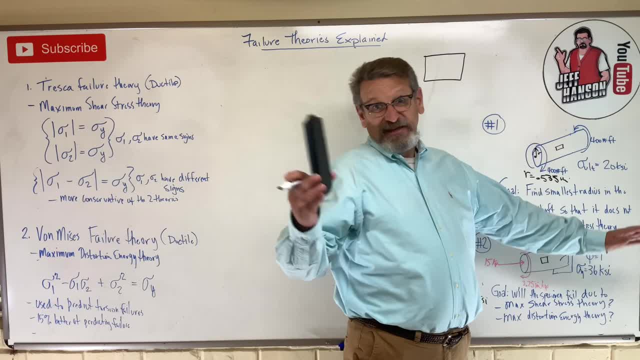 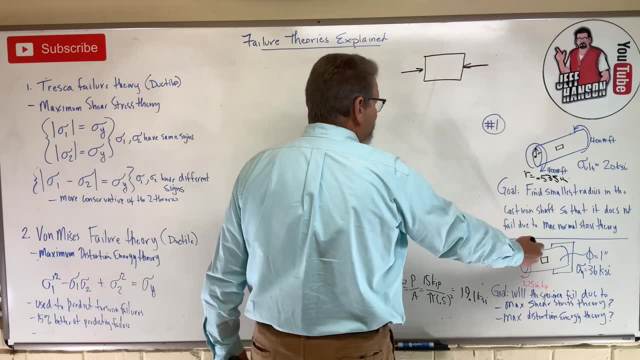 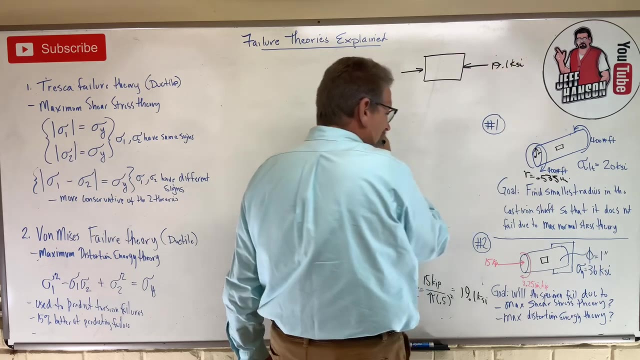 because guess what Sigma yield that I'm going to compare it to it's in KSI. so I'm kind of happy with that. So here's what I've got. If I'm that stress element right there, whoop, here I am bigger. I have 19.1 KSI on me. okay, Now how much do I have any shear on me? 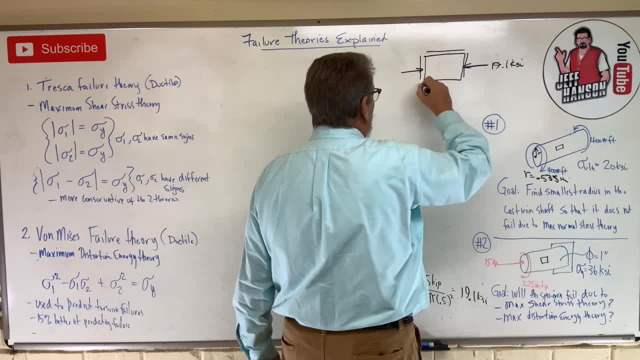 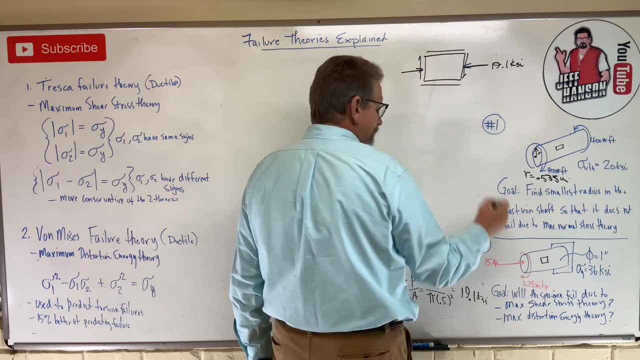 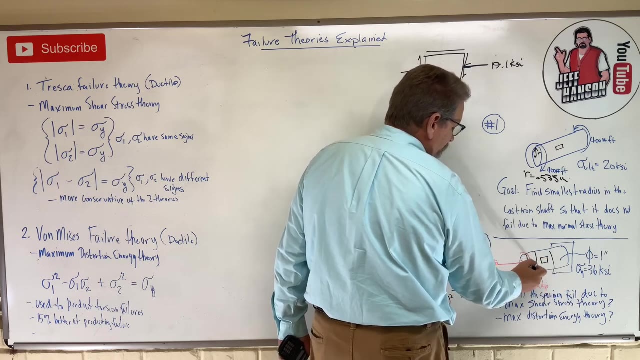 right, Do I have any of this business going on? Okay, and again, let's see up down. how do I do that? I break this in half. right, Break this in half. there's the modal stress element. This guy on this side is going down, so on this side it has to go up. On this side. 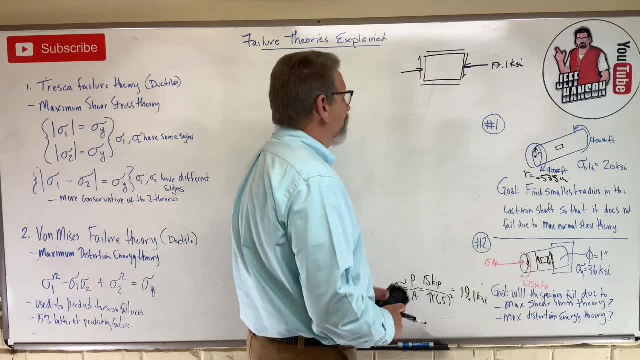 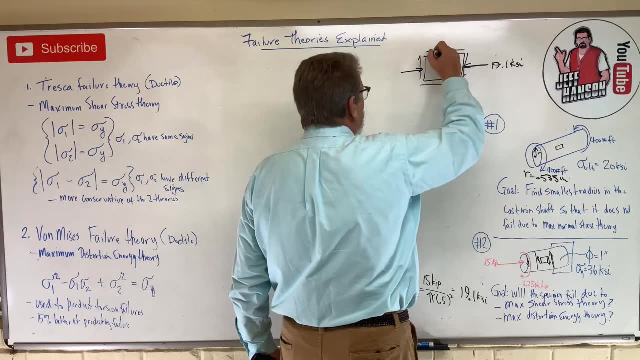 down On this side, up right, I'm just working out the direction of shear. Although it's not important on this problem, it's just good practice to figure out the correct direction of shear, So that little stress element would look like that. right, There's a little stress element A. 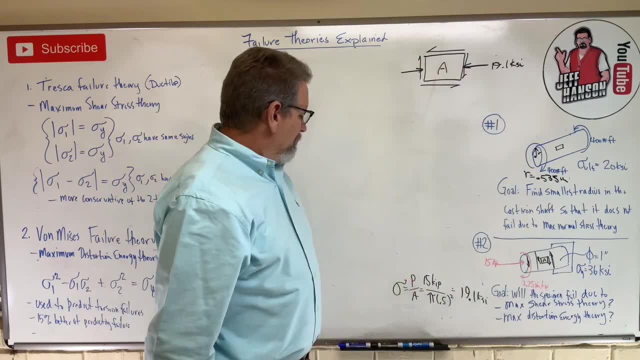 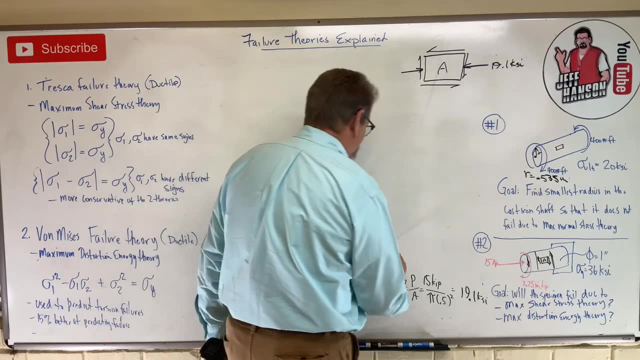 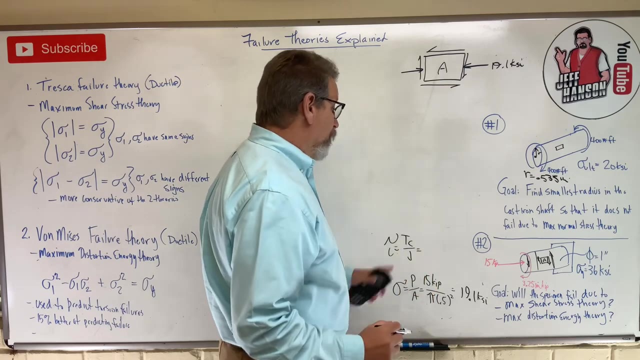 and there's stress element A. Well, isn't it, gang? We got it, though We're almost there. So let's figure out. what is that? tau, So tau. here again, this is a TC over J, isn't it? Okay, the torque: 3.25 inch kips. 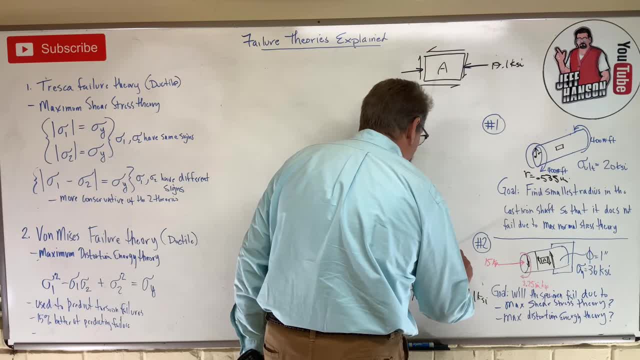 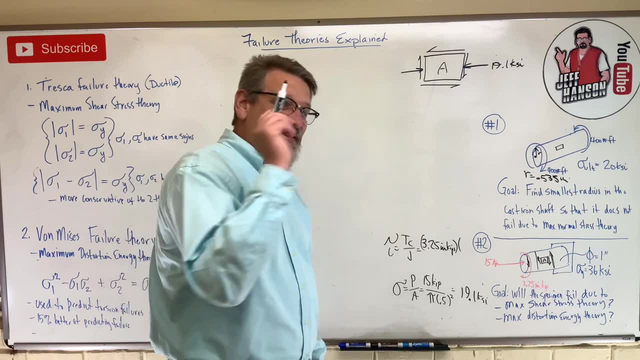 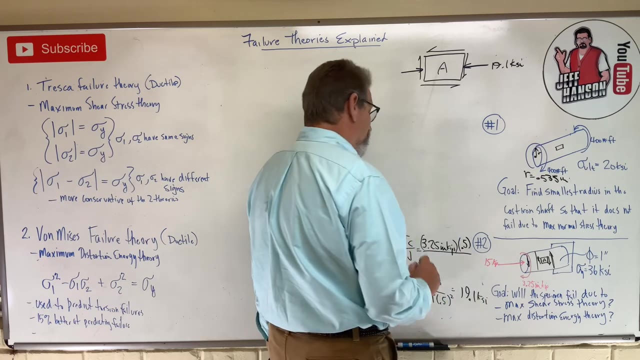 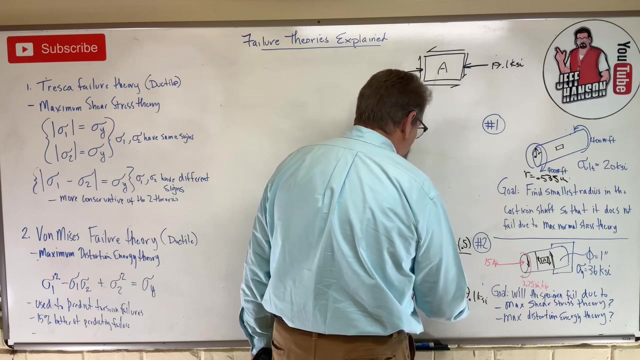 3.25 inch kips. okay, times C. What is C? The distance from the neutral axis to the outside of the part, that's 0.5.. 0.5 divided by J, which is pi over 2 times R to the fourth. okay, And that's inches to the fourth. 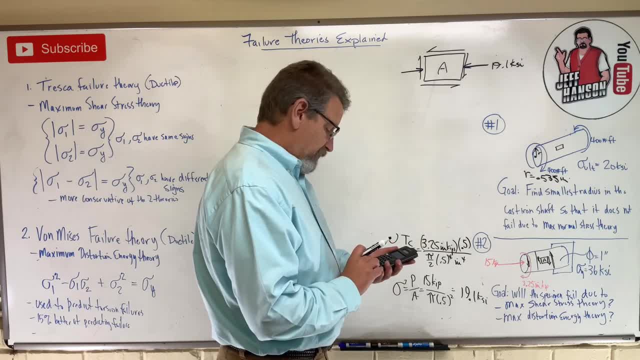 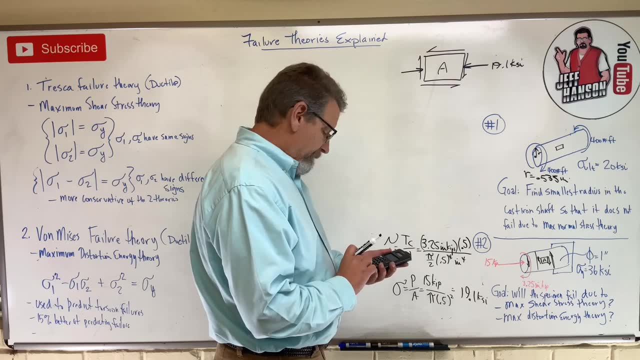 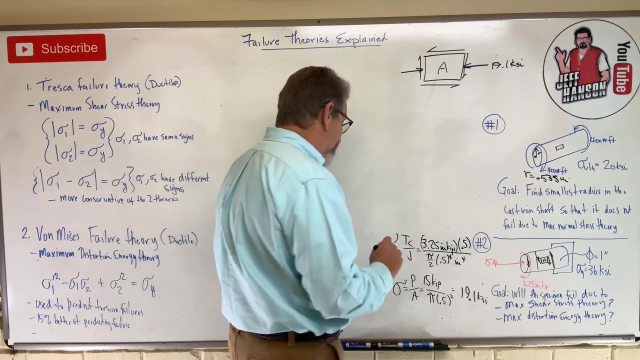 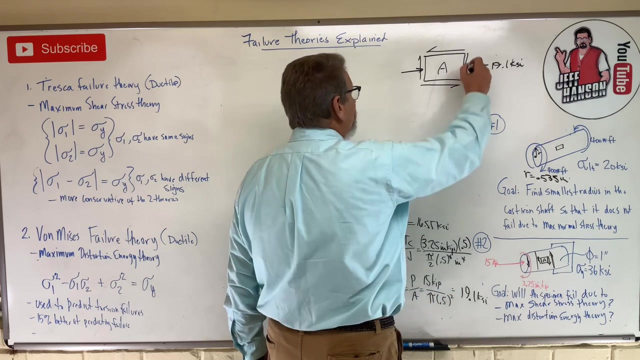 Okay, let's see what that gives us. So 3.25 times 0.5 equals divided by 0.5.. 0.5 to the fourth equals, divided by parentheses, pi over 2. 16.55.. So all that is 16.55.. And that also KSI. Okay, 16.55, KSI. okay, You with me so far. 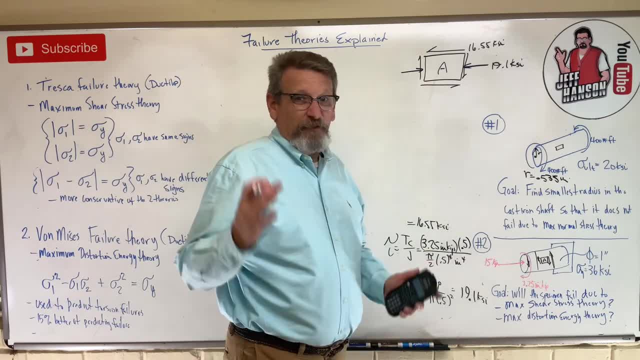 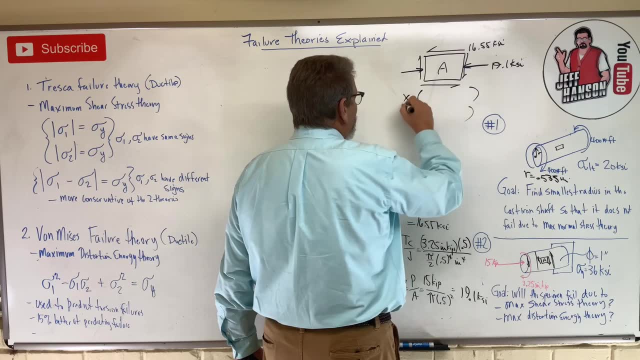 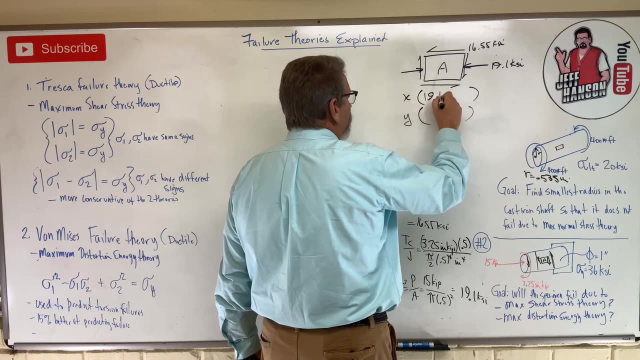 Combined load problem. creative stress element. From my stress element: create a Morse circle. okay, So I need two coordinate points, right, Here's the X face, there's the Y face. okay, On the X face, what do I got? I got 19,, 19.1.. 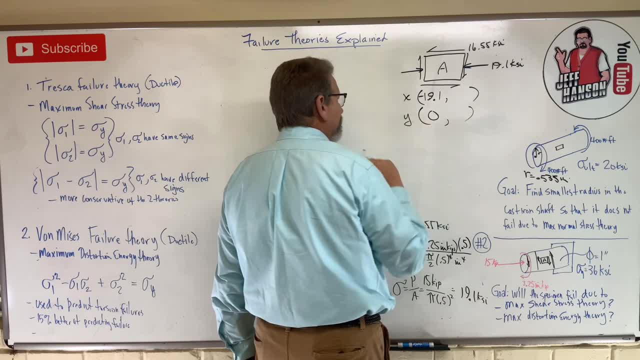 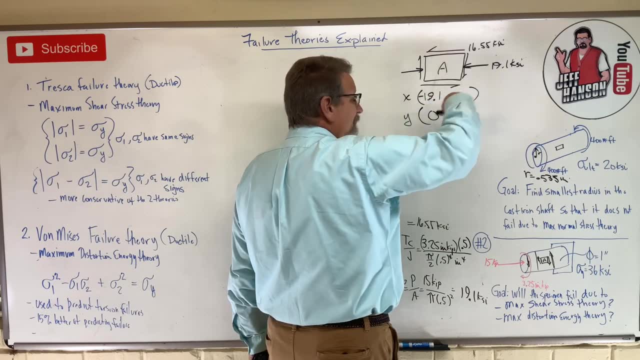 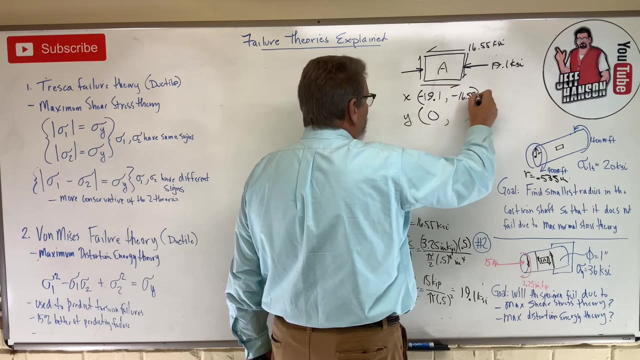 Oh, but it's negative. On the Y face I got. I got 0.. On the tau on my X face over here it's rotating me negative right. So clock above: this is going to be negative 16.55, and this is going to be positive 16.55, okay. 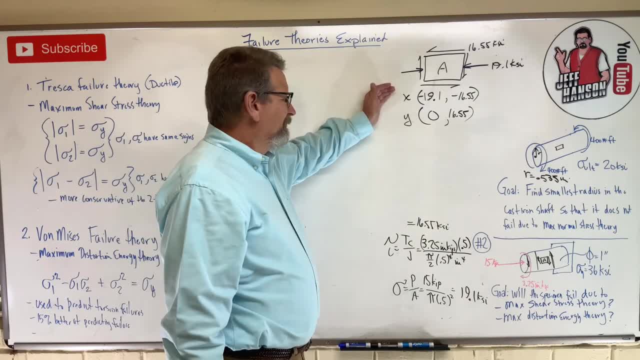 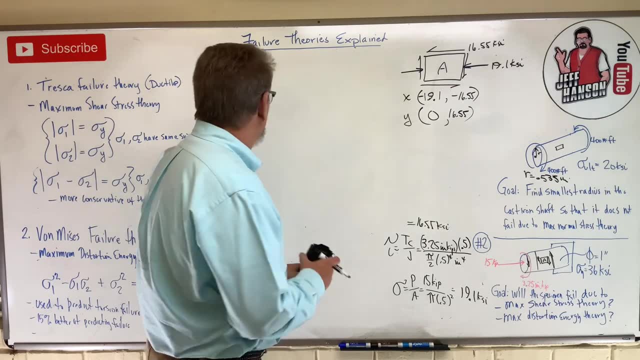 Y'all remember how to do that. We've there's a million Morse circle problems I've got on here, So you go back and review that if you're lost there. Okay, let's, let's plot these, Let's plot them. Here's my Morse circle. okay, Here's tau. 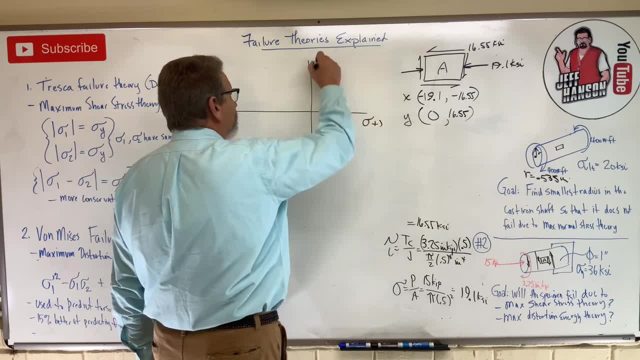 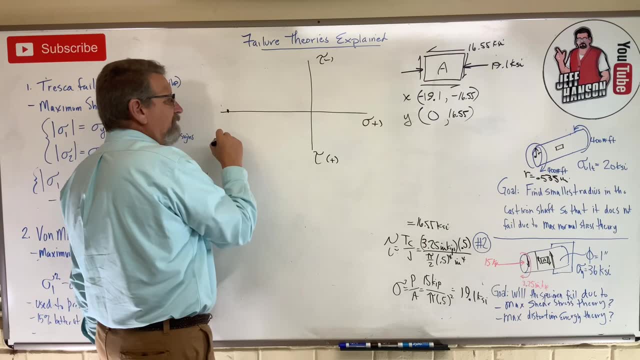 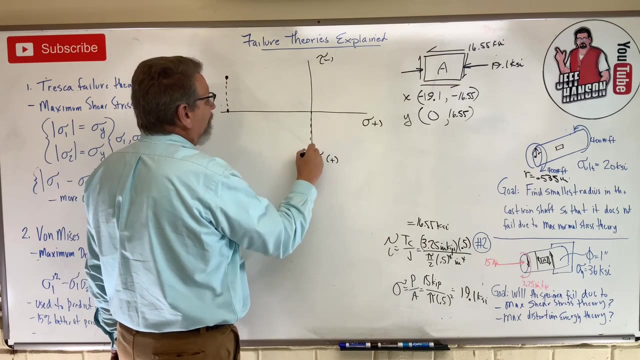 sigma. this is positive, this is positive, this is tau. negative. okay, And the first point is negative 19.1, which is there, and negative 16.55, that's there. The next point is 0 and negative, which is there. So there's my deal here. 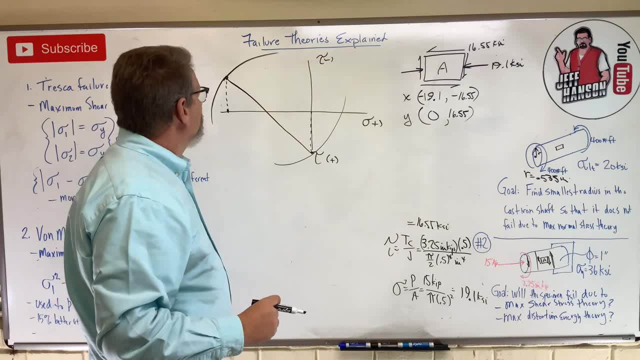 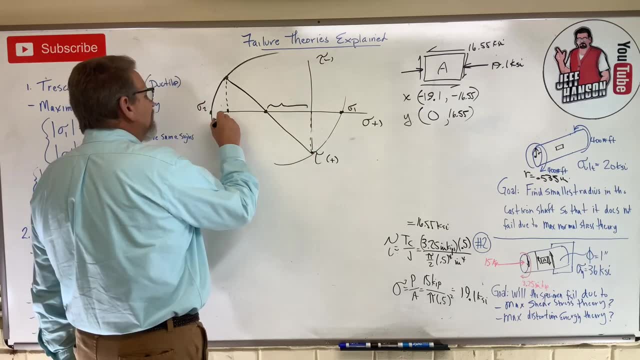 Okay, imagine that making a whole circle there, okay, So what do we got? Let's see from here to here. so, on our circle, this is 19.1, and this height here 16.55,. this height here. 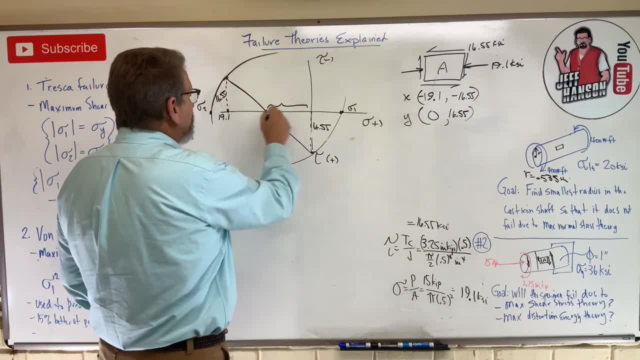 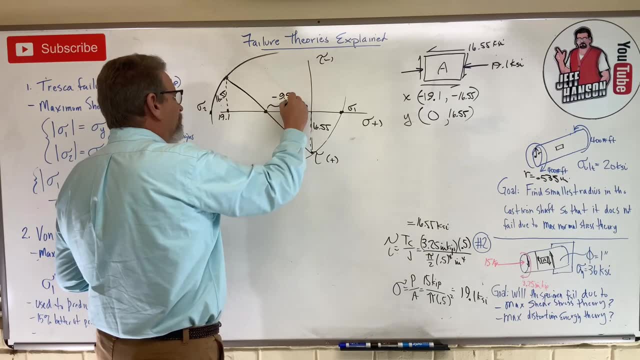 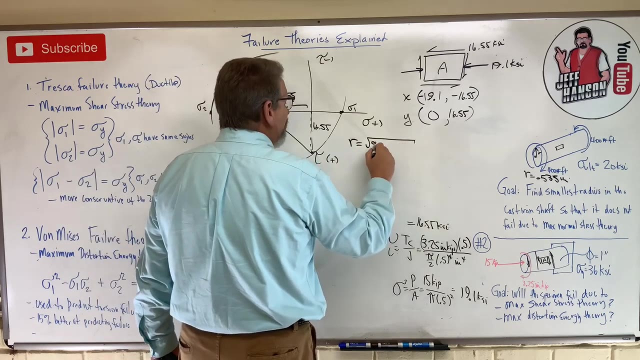 16.55,, which means that this distance here it's got to be half of 19.1,, doesn't it? Which is negative 9.55,. okay, So let's calculate our radius, which is 9.55 squared plus. 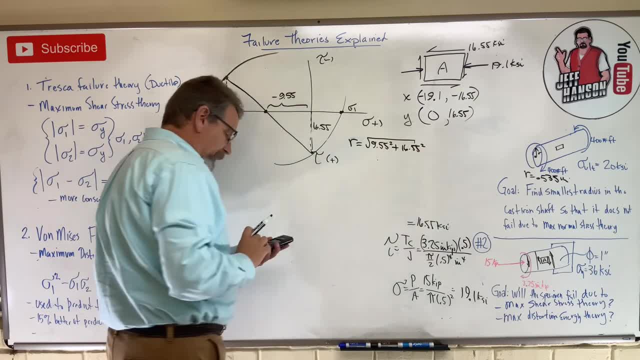 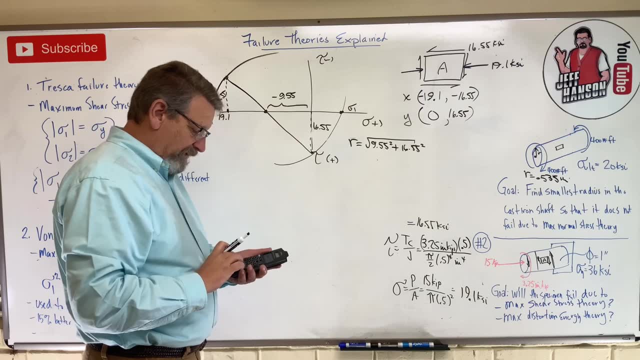 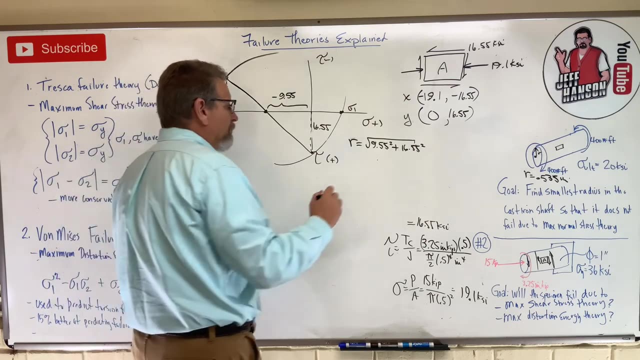 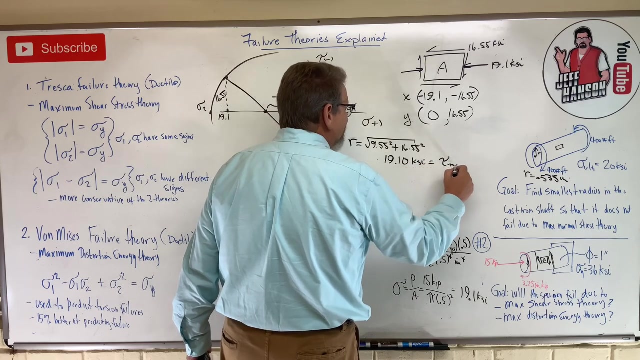 16.55 squared square root. 9.55 squared plus 16.55 squared equals second square root. second answer equals 19.10, 19.10 KSI. And guess what? That's tau max, isn't it Okay And remember. 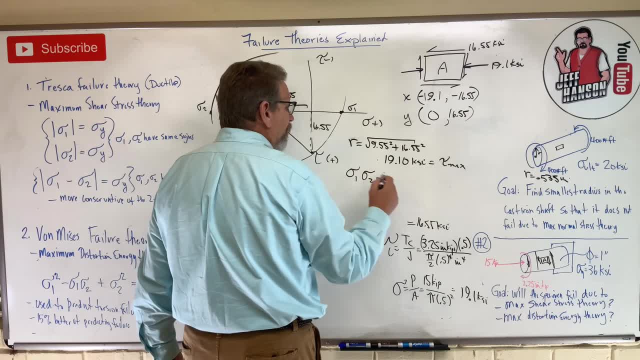 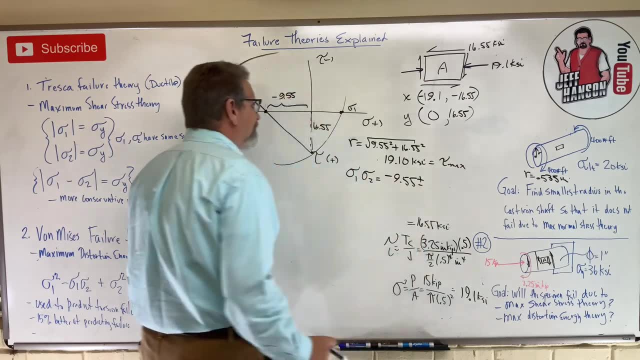 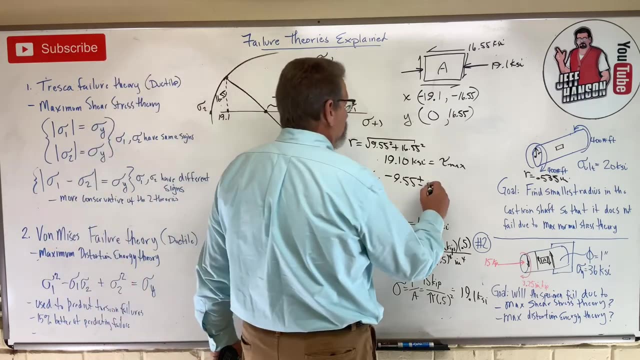 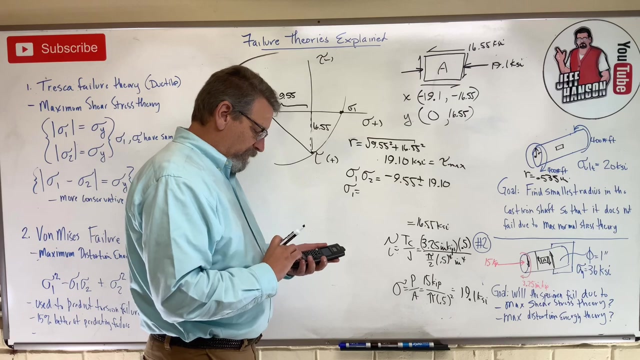 sigma 1 and sigma 2, are equal to what The center point, minus 9.55, plus or minus right. Sigma 1 is plus a radius, sigma 2, minus a radius right, So 19.10.. Okay, so here we go. Sigma 1 is what 19.10 minus 9.55,. 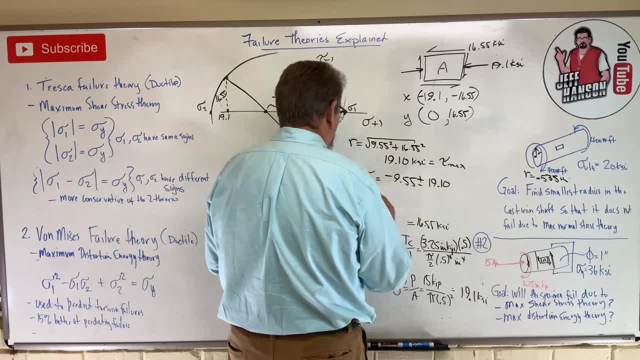 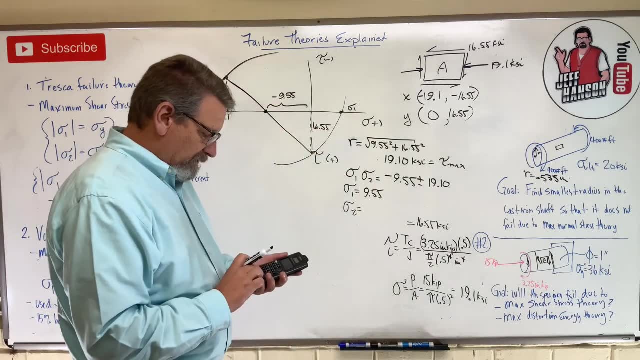 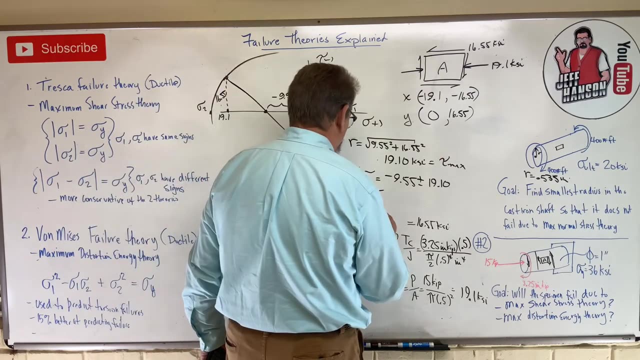 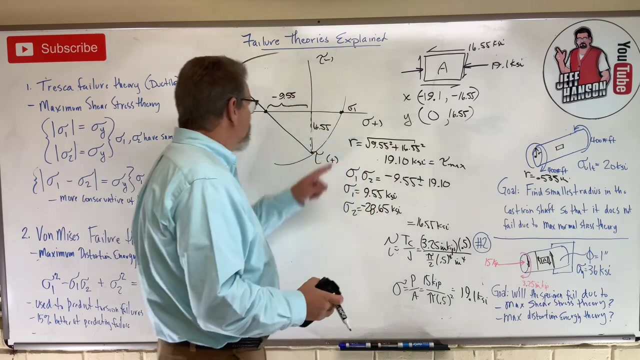 9.55.. Sigma 2, sigma 2 is what 19.10 plus 9.55 equals 28.65.. That's KSI, that's KSI, but this one is negative. right? Sigma 2 is negative, isn't it Okay? 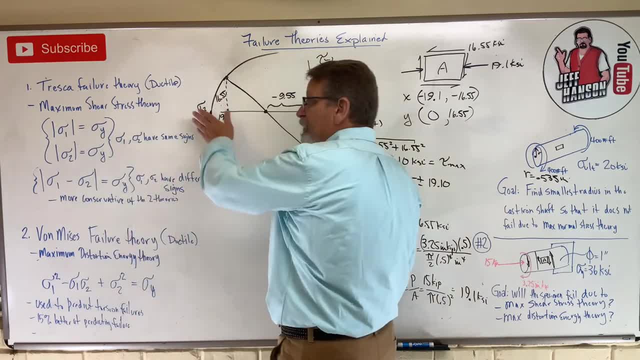 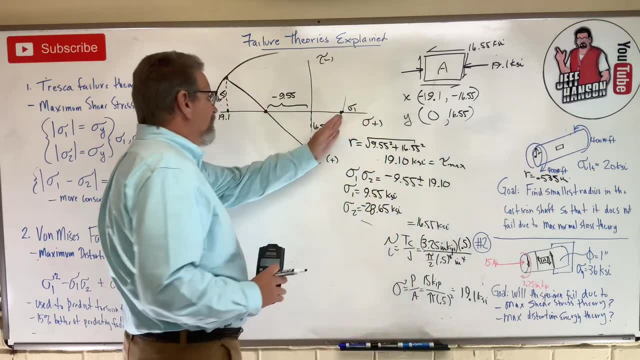 All right, here we go. Let's use our maximum shear stress theory. Bam, that's what they want to do first. right, Do we have the same signs? Well, sigma 1 is positive, sigma 2 is negative. No, we don't have. 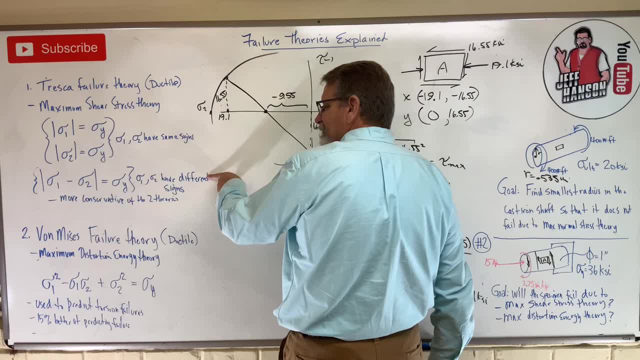 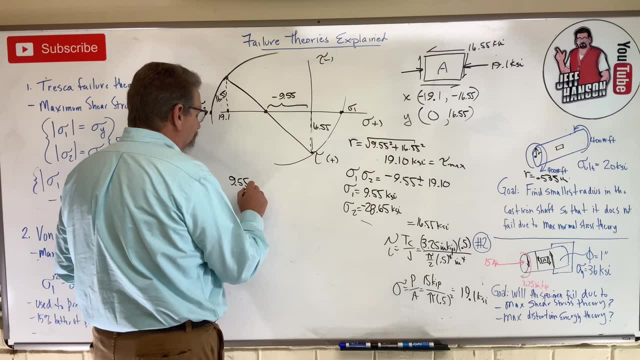 the same signs. So then, what does that mean? We need to use this guy. okay, Sigma 1 minus sigma 2.. So sigma 1, 9.55 minus sigma 2 minus 28.65.. And we're going to compare that to what. 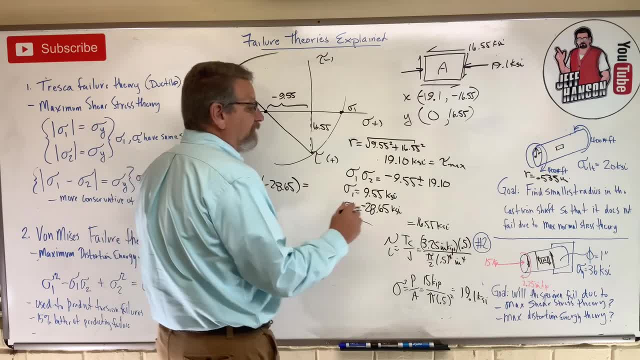 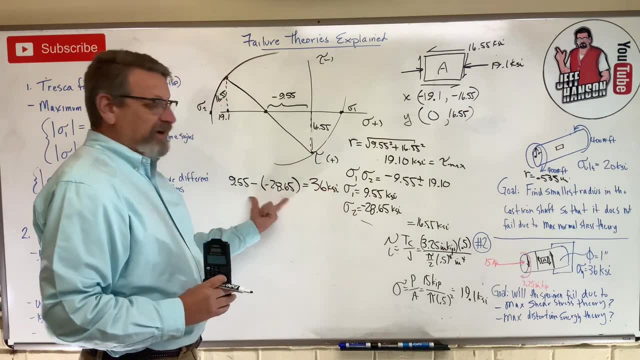 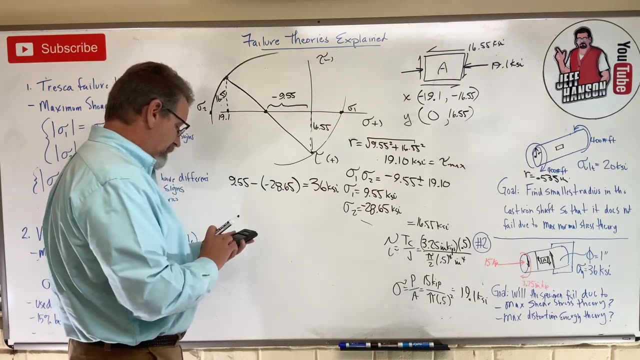 To sigma yield, right, Sigma yield is: was that given up 36.? Okay, remember, if this side is bigger than 36, we got a failure. If this side is smaller than 36, we're okay. Okay. So here we go Now. minus of minus, that's going to be plus, So 9.55. 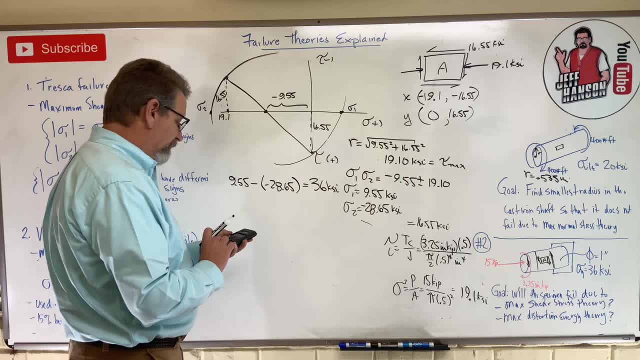 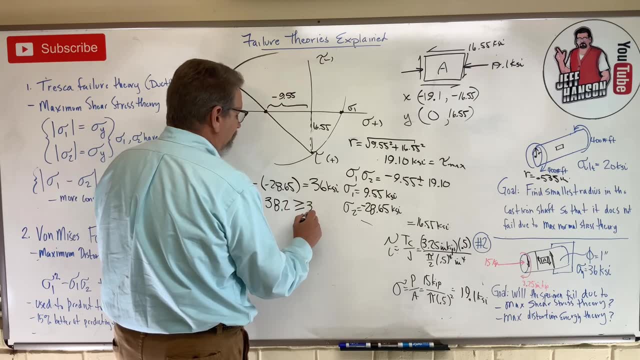 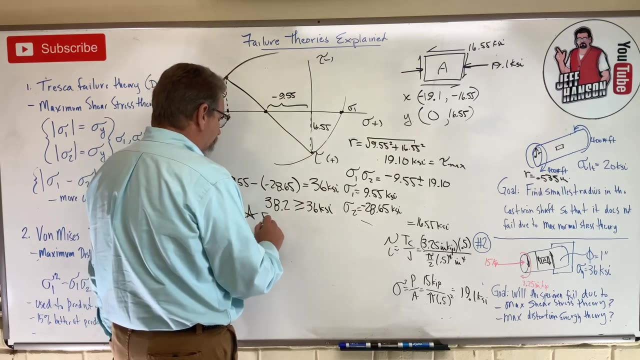 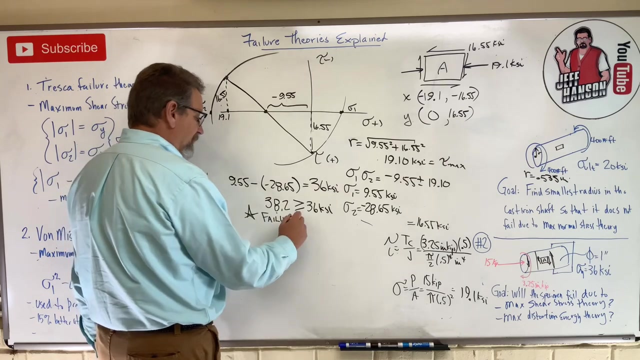 plus 28.65 is 38.2, which is- guess what? Greater than 36 KSI. So what do we got here? Wah, wah, wah. This failure theory is predicting that that thing is going to fail, right, It's. 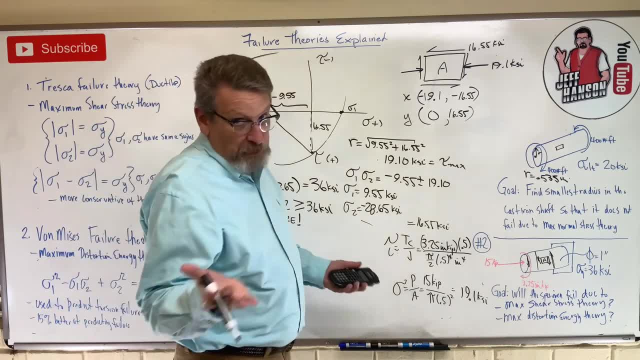 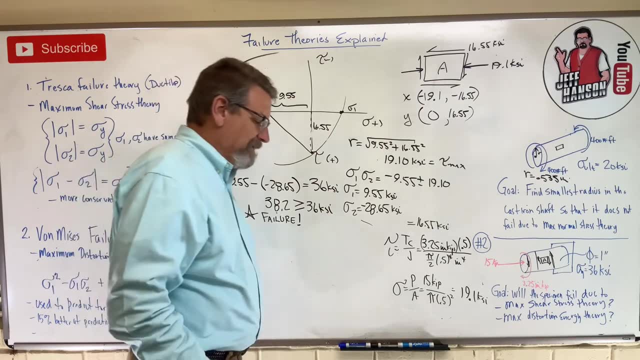 going to fail. Now it's pretty close. right, It's pretty close. On these ones that are pretty close, you might want to check it one more time with the other theory and see what it says. okay, So let's try the other theory, which is the von Mises failure theory or the maximum distortion. 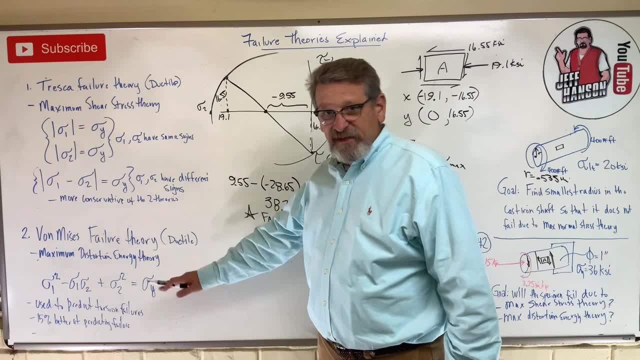 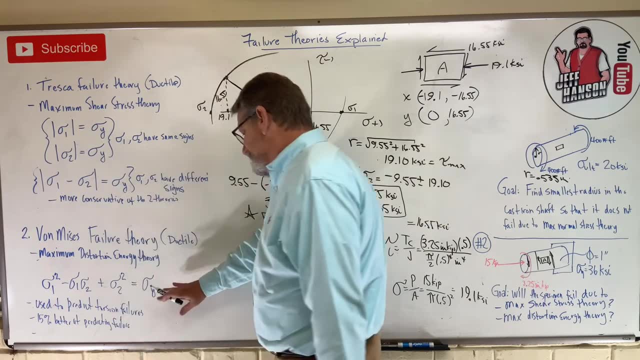 energy theory. It's just sigma 1.. Sigma 2, we already got that, don't we? There's sigma 1 and sigma 2 right there. okay, Now we're going to take that and compare it to the yield and see if it fails. So let's do that. 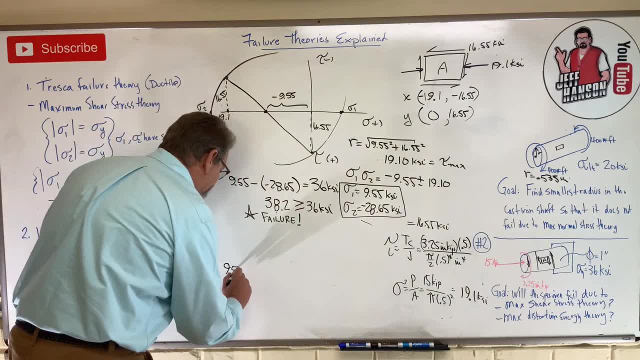 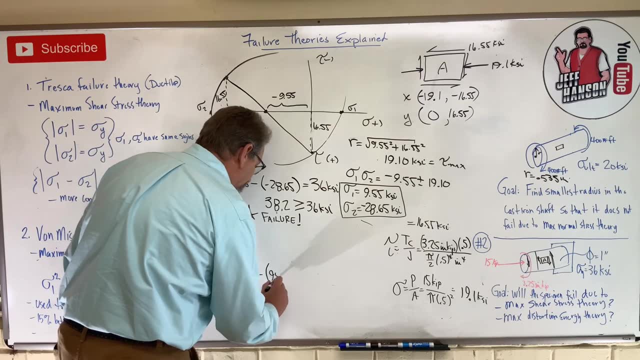 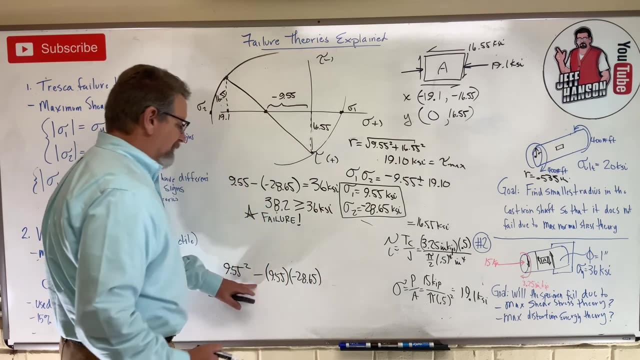 So sigma 1 squared is 9.55, squared minus: okay sigma 1, 9.55 times sigma 2, negative 28.65.. Again, minus and a minus. It's going to turn out to be minus, So we're going to take that and 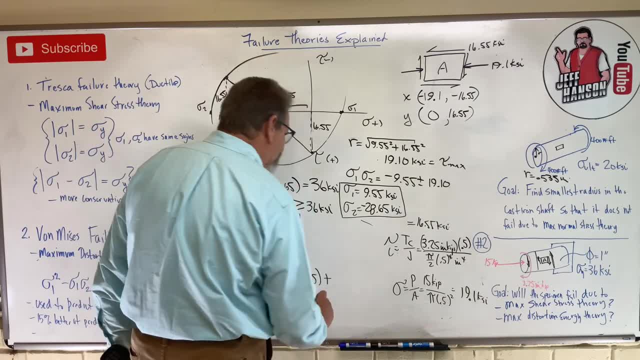 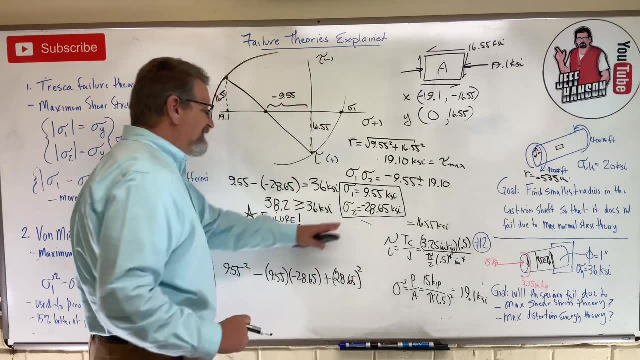 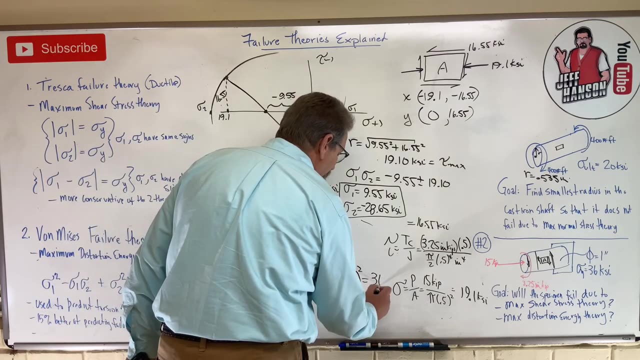 turn that into a positive, plus sigma 2, 28.65 squared, But it's negative, I'm squaring it. okay, Get off me. Gah Equals: here it is 36 KSI. okay, So is this failure? is this going to? 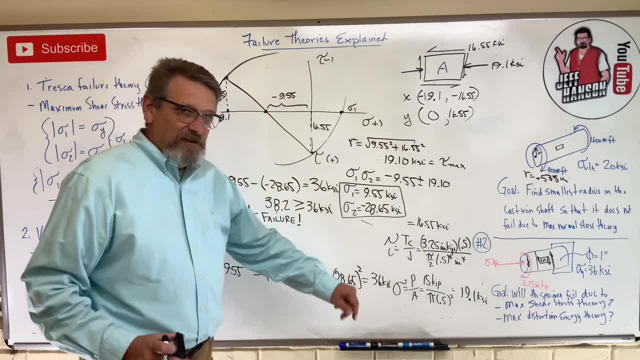 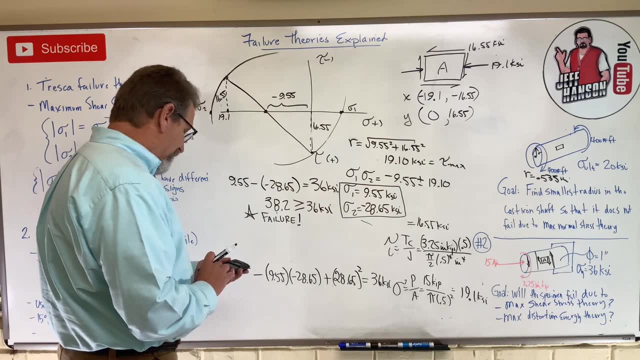 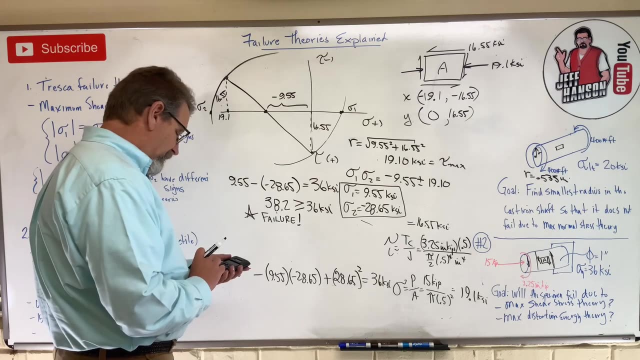 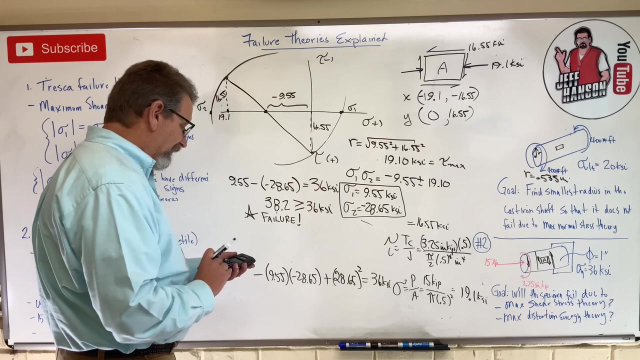 be bigger than 36?? It's going to say fail. If it's less, we're okay. All right, So let's go. 9.55 squared plus 9.55 times 28.65 plus 28.65 squared equals 1185.. Oh yeah, I forgot one. 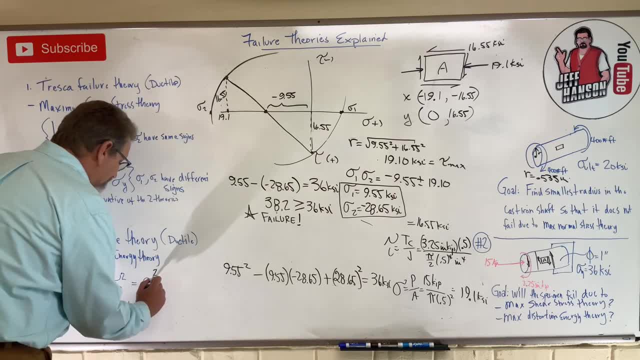 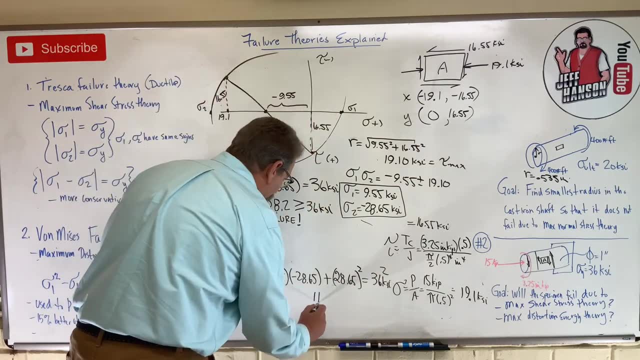 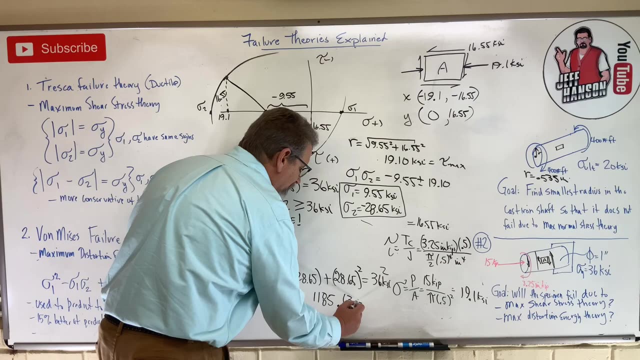 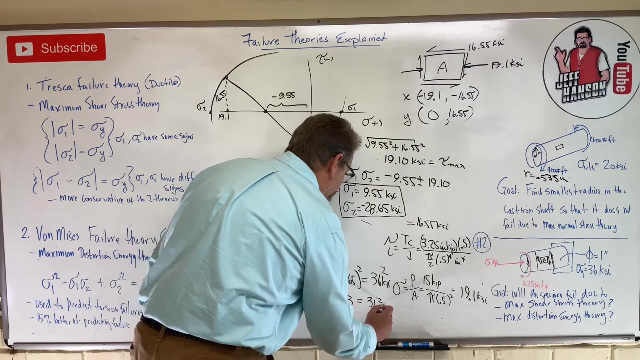 thing, I forgot something. This has to be squared right there. right, This has to be squared right there. So 1185.. Oh my gosh, Hanson, come on. 1185.63, okay, is equal to 36 squared, So let's just. 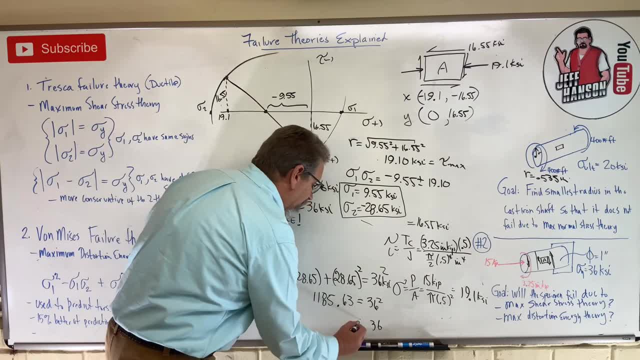 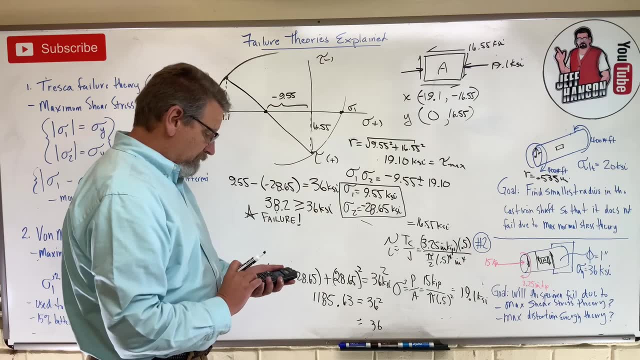 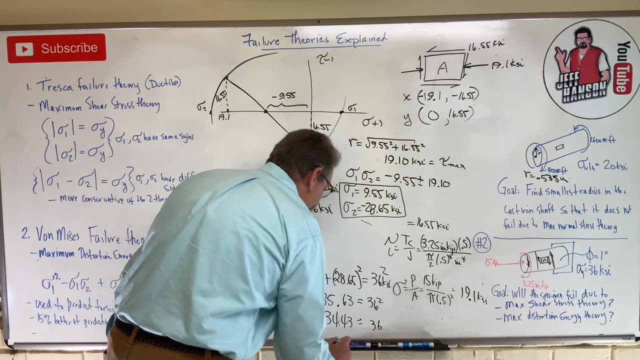 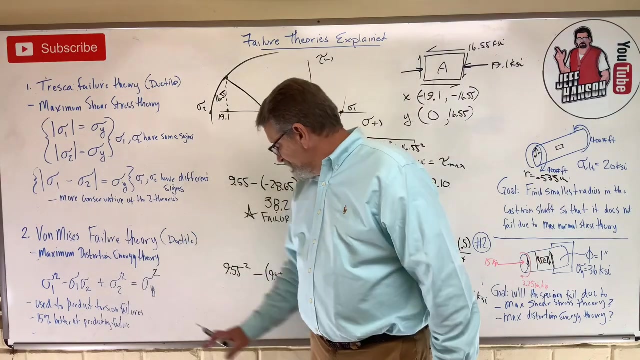 take the square root of both sides. So 36 over here. And what's the square root of that guy? Second square root, second answer, equals 36.43.. Guess what That number is less. So this theory over here, this one over here, says: 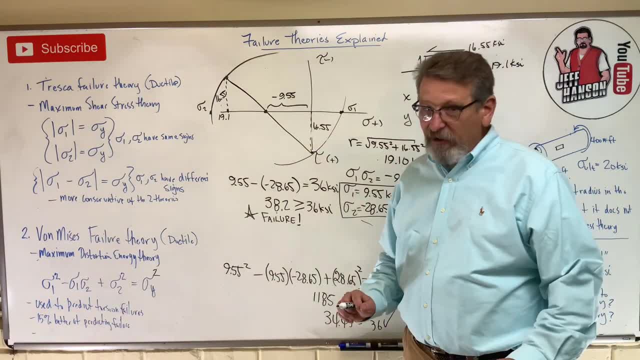 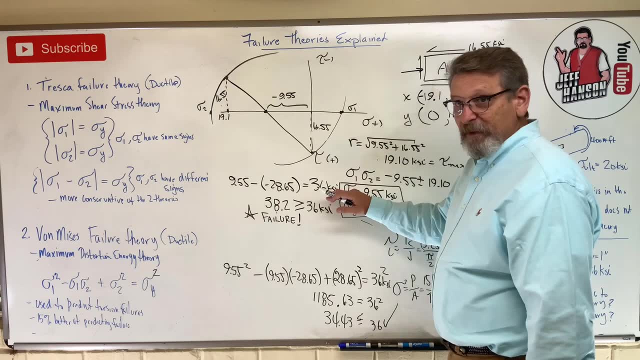 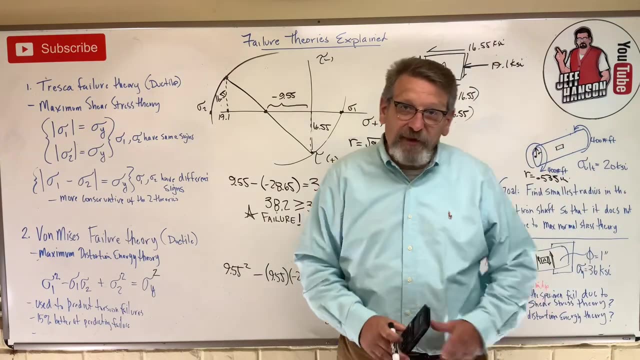 hey, it's okay. Just barely, but it's okay. This theory up here says we're going to have a failure, So be careful. This is more conservative. Remember: this is more conservative. This is 15% better, especially on torsion problems, which is what we have here, right? 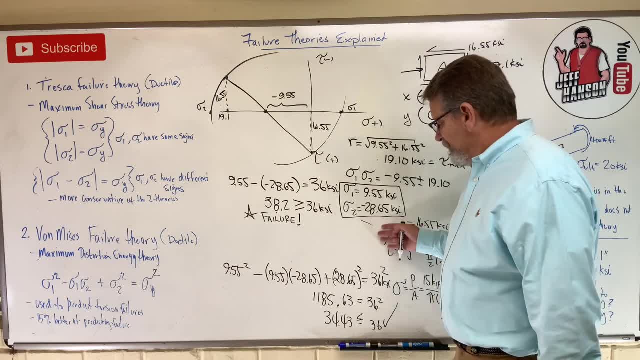 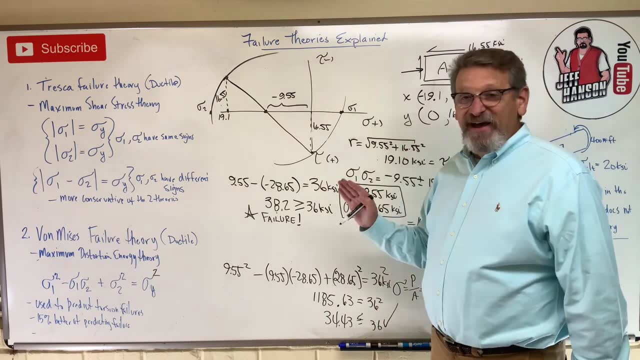 Now again, if you're my engineer and you're working for me, I don't want you to be this close to the limit. I need a little factor of safety in here, right? But anyway, that's how you use these theories, okay? All right, I hope this clears up some of your muddy thoughts. See you next time.